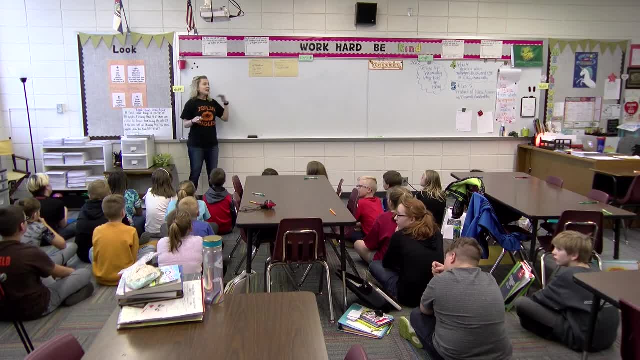 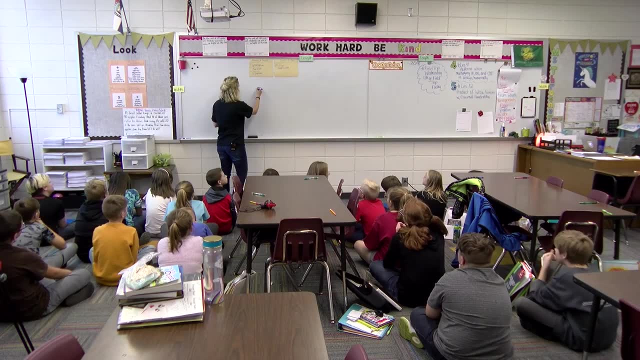 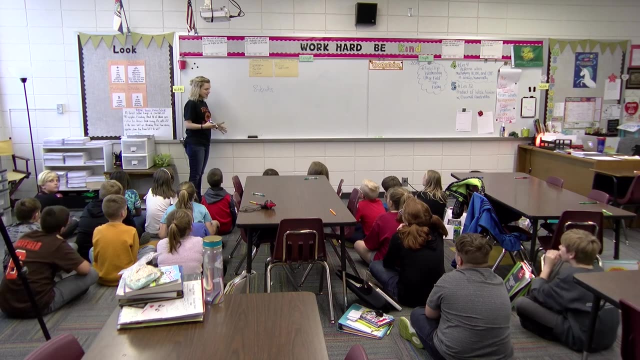 our brains. Now, thinking back to unit one: concepts. Now, that's been a while, Would you guys agree with me? Whew, we've done a lot of math. What if I provided you with a unit form of eight-tenths? How do I write that as a decimal and how do I say it, Thomas? 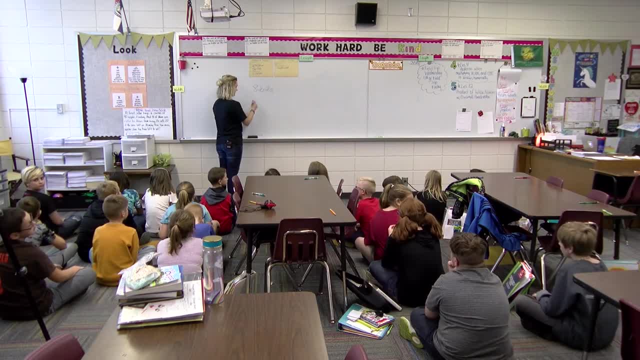 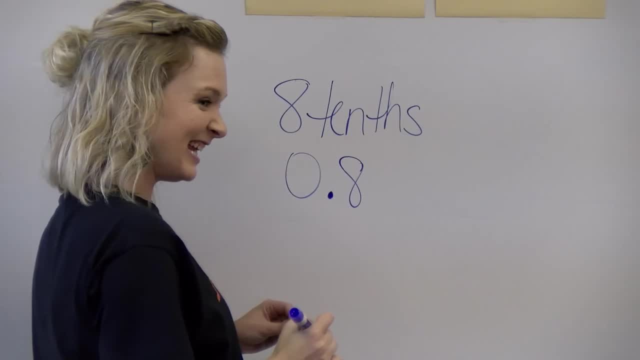 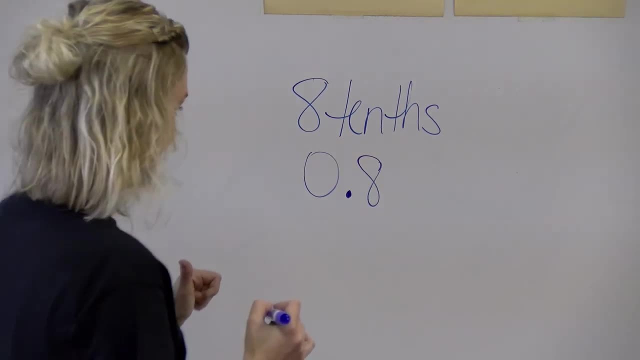 Zero, nine, eight. We don't call that point. What do we call it bud? We call it zero and eight-tenths. Thank you so much. And the reason we call it, that is because, and the reason we call it, that is because, and the reason we call. 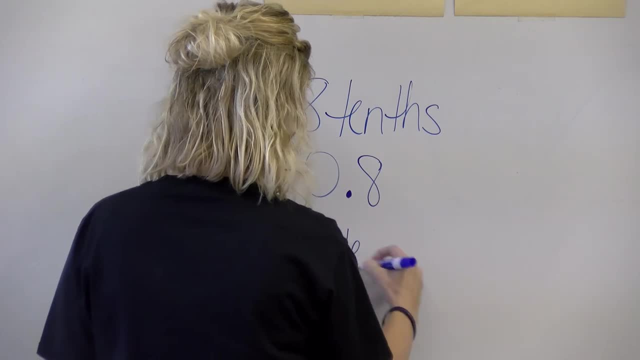 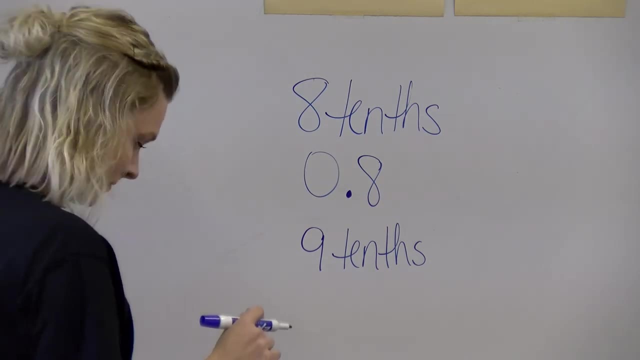 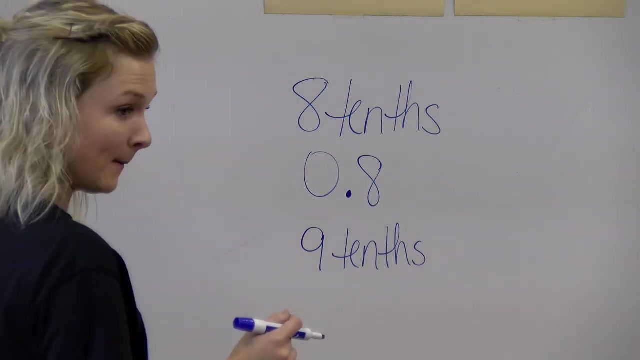 it. that is because zero is in the one place. so if you have nothing in that place, you put a zero in that place. you don't have to, but you can if you want to. The placeholder right And when you so, when you're pronouncing it, you got to get in that right place value. 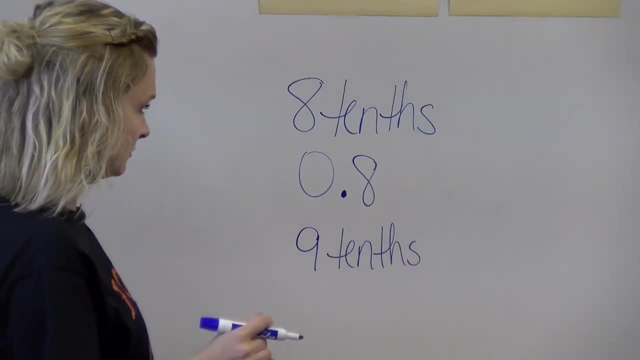 Exactly. We want to land in the tenths. So let's do that same thing with nine-tenths. How do I say it correctly? Nine-tenths, nine-tenths, nine-tenths. Okay, there's nine-tenths and then? I add them into the class Nine-tenths, nine-tenths, nine-tenths, nine-tenths, and then I add them in nine-tenths, nine-tenths, nine-tenths, nine-tenths. So that's what we're going to do. 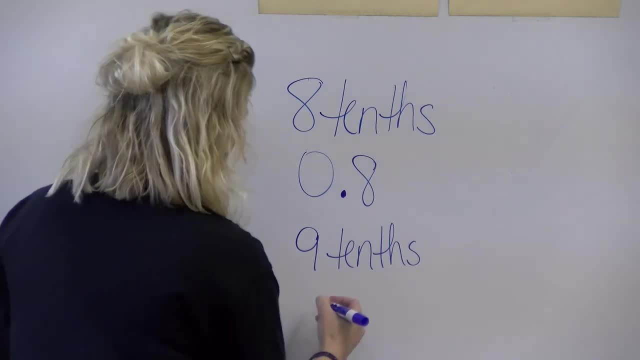 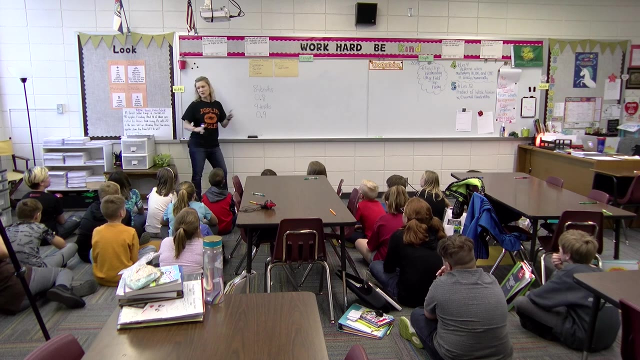 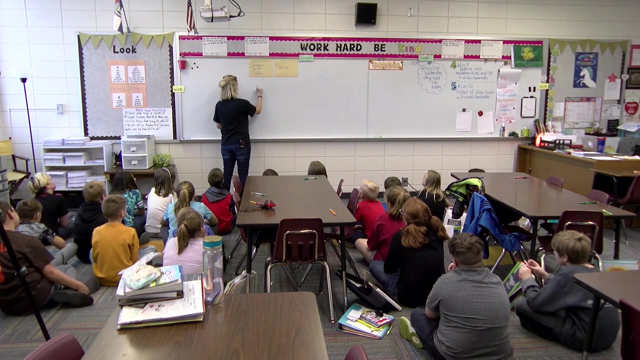 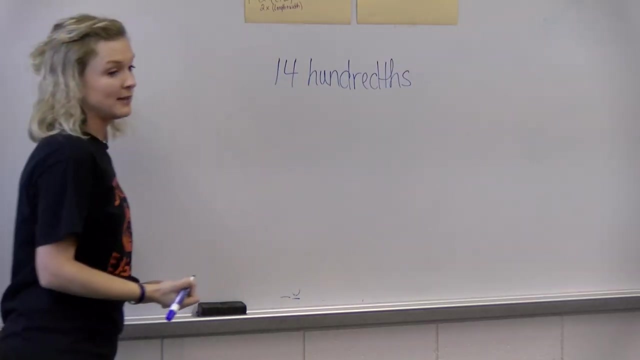 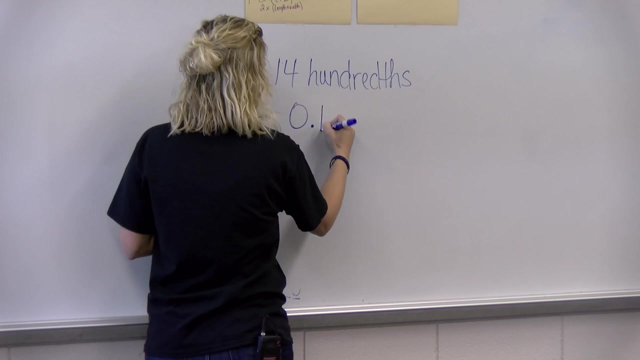 say it? and how do I write it as a decimal? Olivia? how do you say it? thank you, but let it. let me change it. so we were on tense. now we're jumping to hundredths today as a quick review. fourteen hundredths- how do I write that as a decimal? how do I say it? Cole, zero. 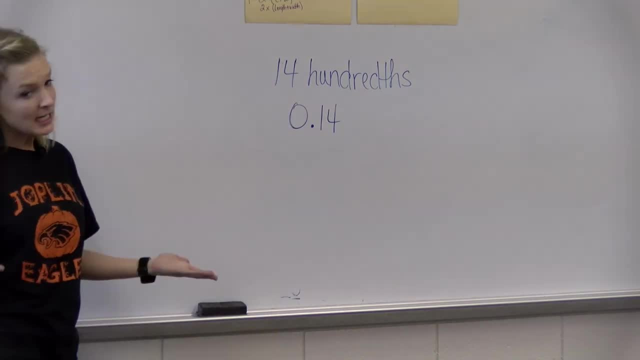 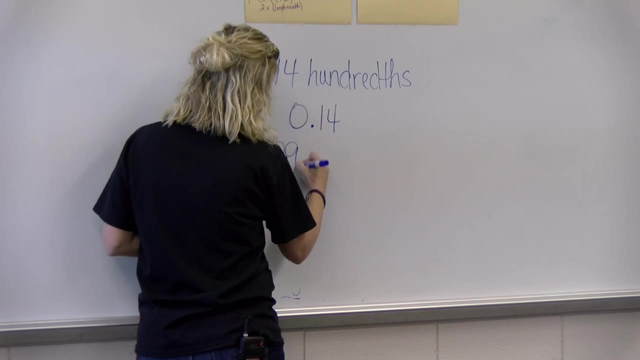 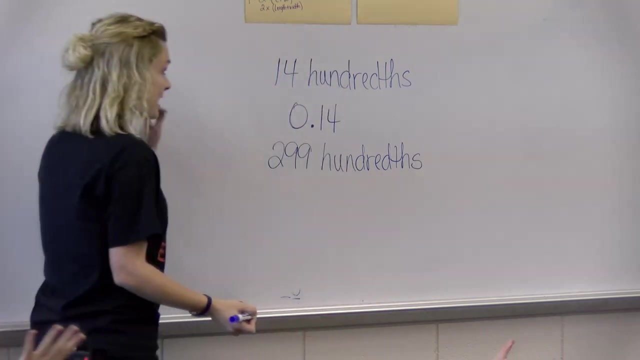 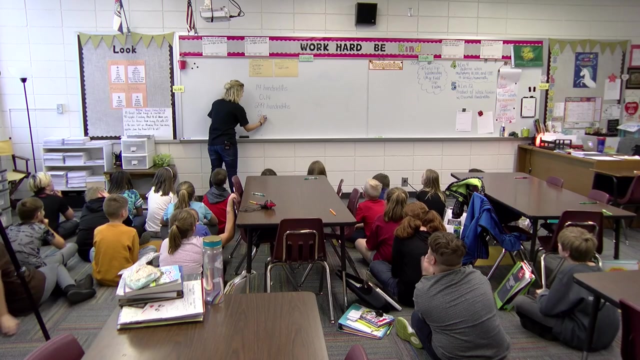 and fourteen hundredths. did I write it correctly? did I land in the correct place value? oh, that was tricky. now I'm gonna throw a challenge to you. two hundred ninety nine hundredths, how do I write that as a decimal? and how do I say it, Elena, how do you say it? 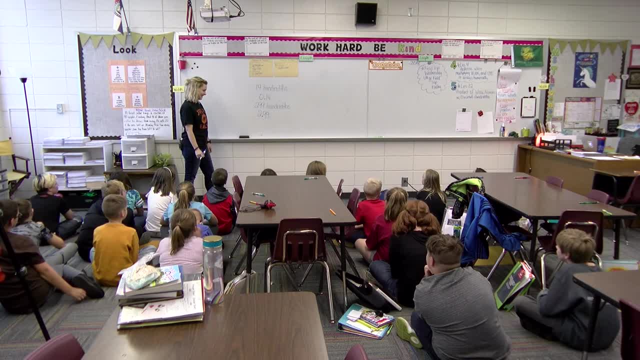 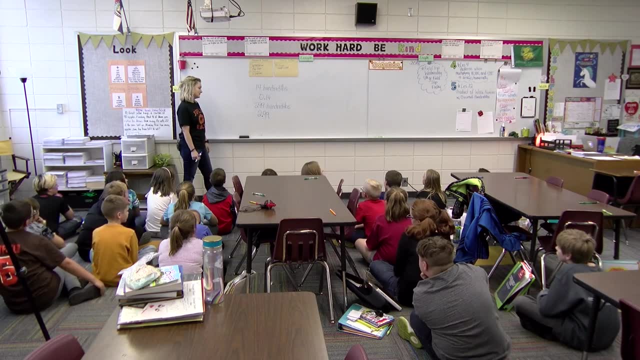 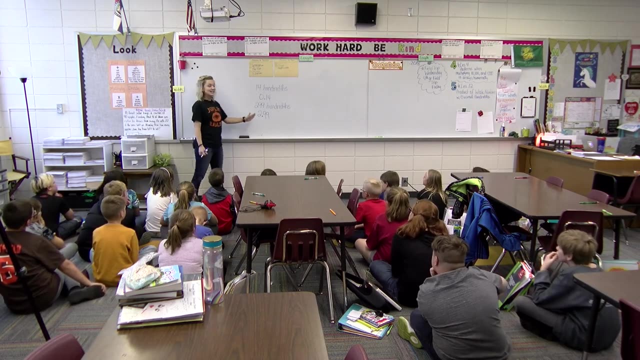 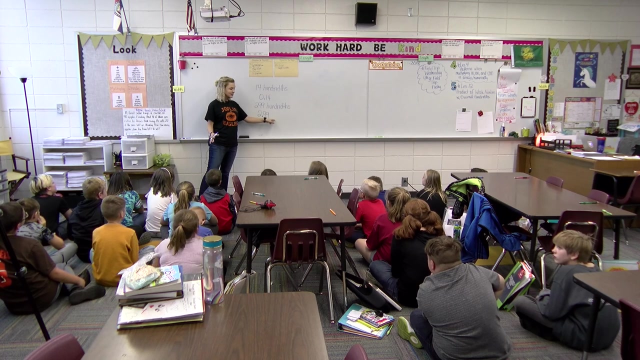 Elena, you're correct. how did you know you needed to kick that two on the other side of the decimal place exactly? did you hear she how she explained that if she didn't push that out to the ones, we would actually be landing over here in the thousands? 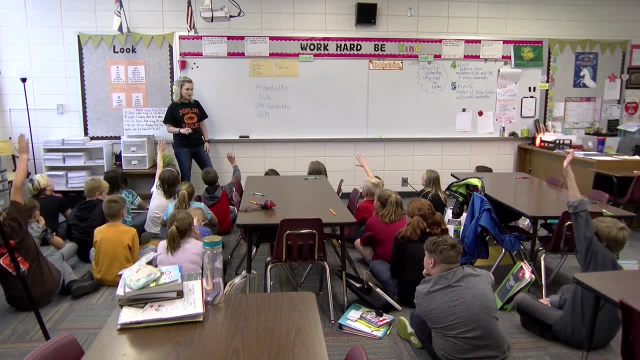 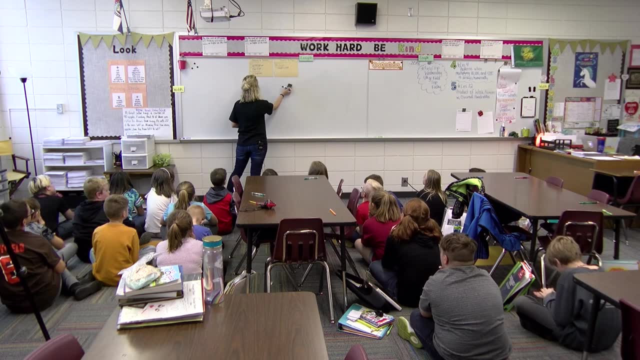 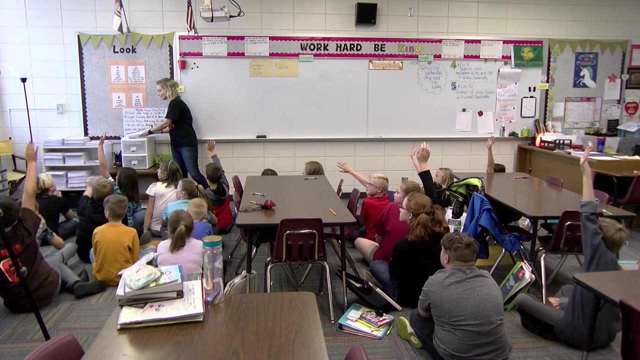 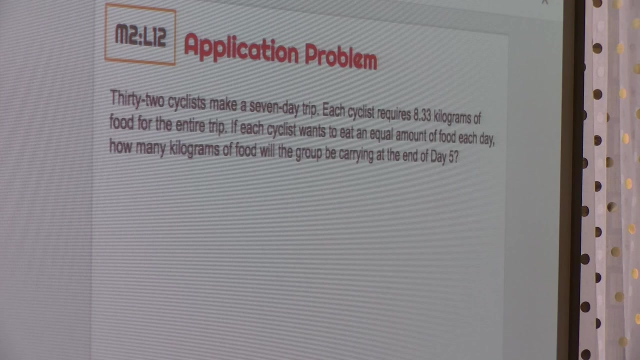 because the hundredths place is how many places after the decimal? Alexis, two way to go. team whoo, throwing a lot at you very quickly. all right now I need someone to read the application problem to us. what does it say, Charles? Charles, make a seven-day trip. each cyclist requires eight and three hundred. 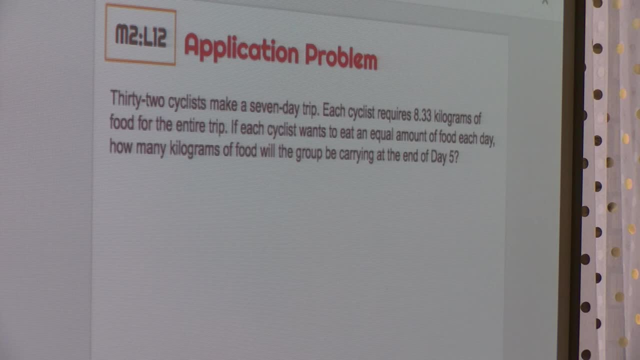 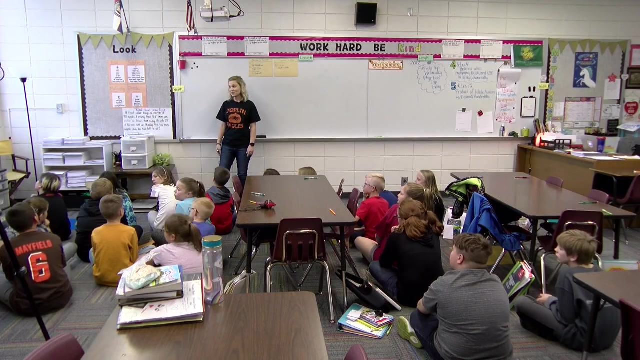 kilometers of food for the entire trip. if each cyclist wants to eat an equal amount of food each day, how many kilograms of food will they eat? how many kilograms of food will they eat? how many kilograms of food will they eat? wow, thank you so much. that said a lot in one word: problem. let's break down what. 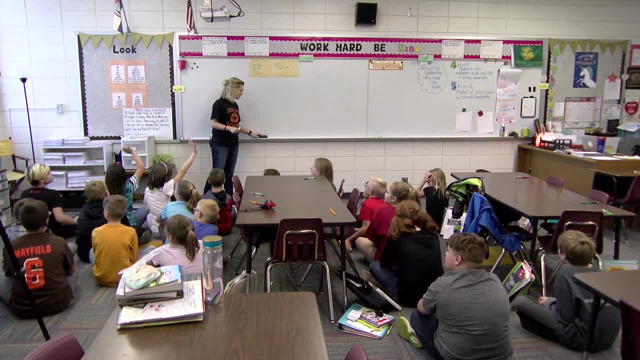 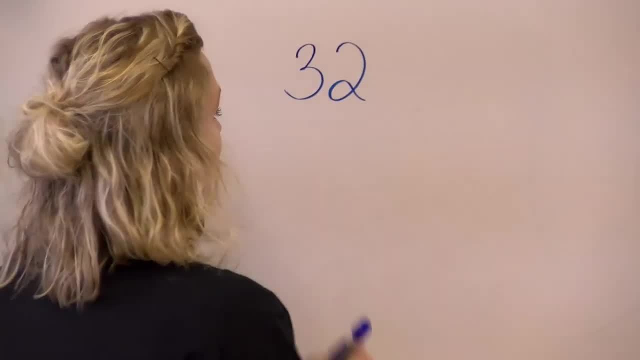 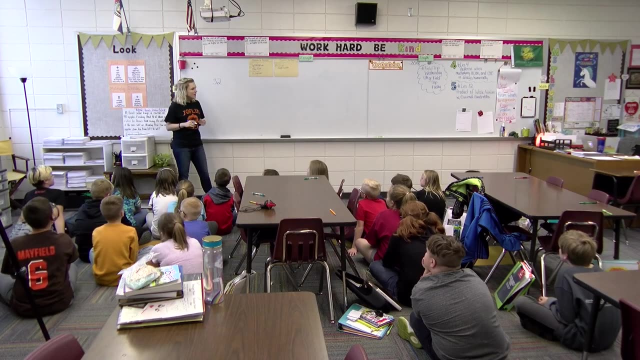 we know someone tell me first of all, how many people do we have going on this trip, Megan? oh, 32, that's a big group. now, a cyclist is just someone who's gonna ride a bike for a very long distance. okay, that's all that means. how long are they? 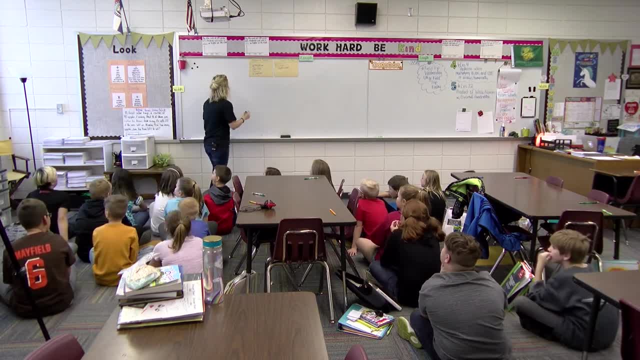 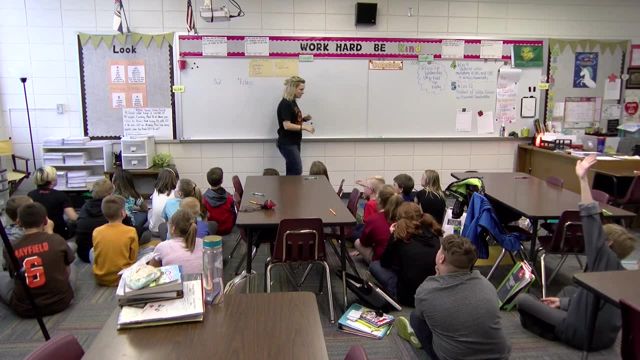 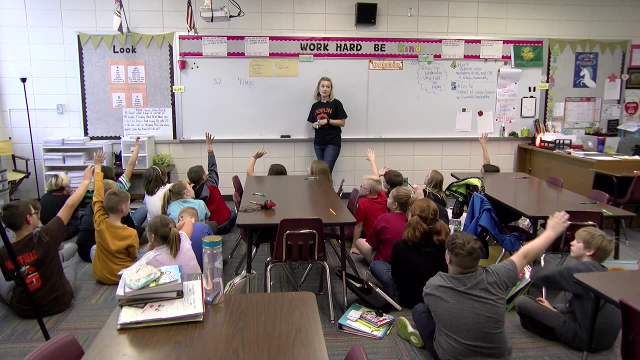 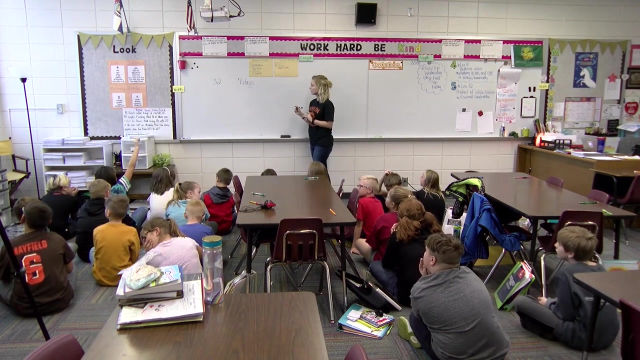 gonna be gone, Ethan, Speaking whoo man, I bet they're gonna be tired. someone tell me how much food to keep up there, herrdy, are they going to require across each who, not each day, but the entire trip. whoo Thomas on, not kilometers, what is it? 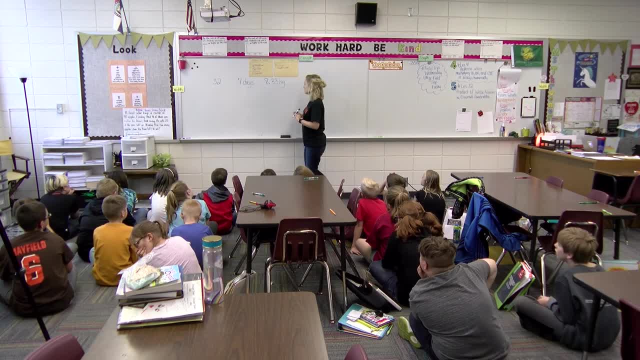 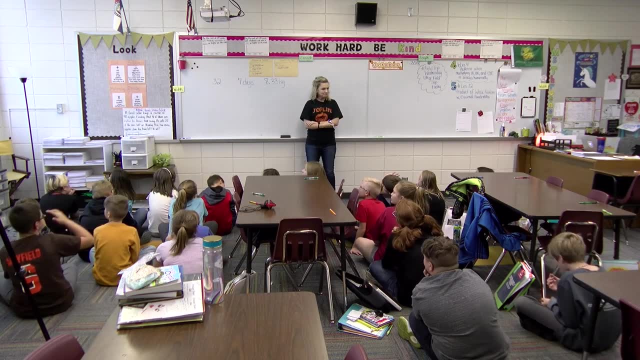 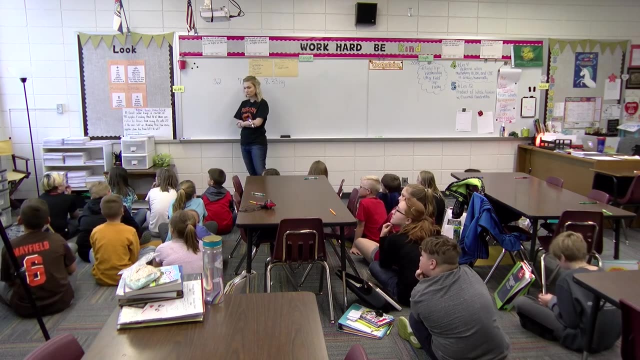 Kilogram. Thank you Sorry, That's okay. It's a quick fix, No worries. So that's for the entire trip. What are they asking us to find, Cole? How many kilograms of food will a group be carrying at the same time? 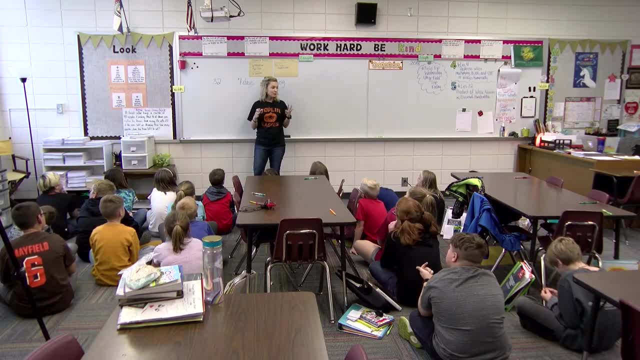 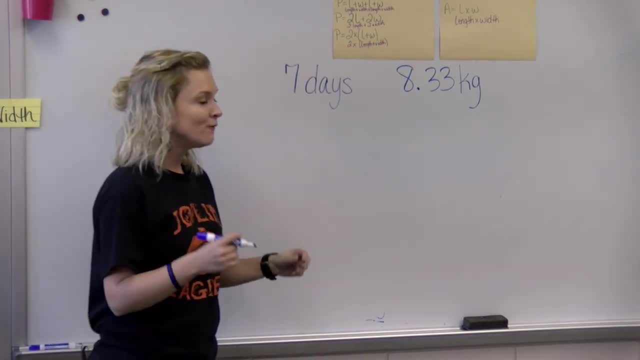 Now Miss T had to break down this problem in three steps. Are you guys ready to work those steps with me? I think we can do it. So someone tell me how much food did we say each cyclist is going to need across their entire trip? 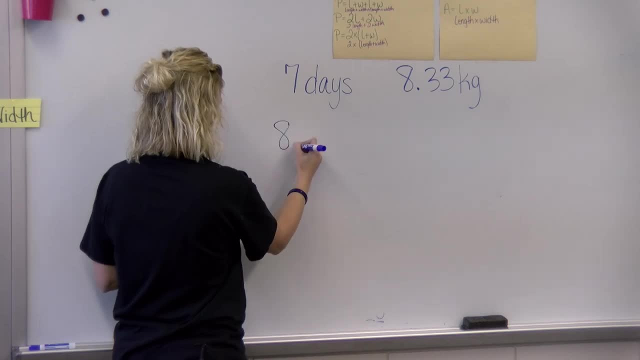 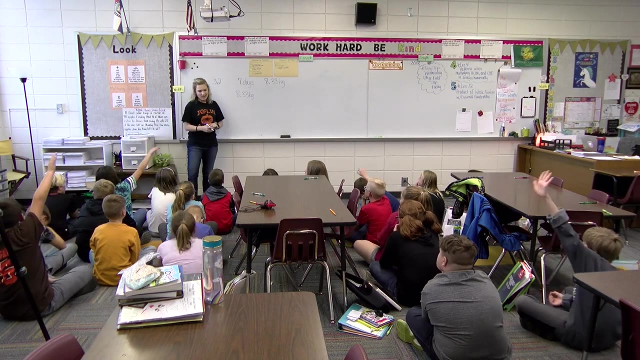 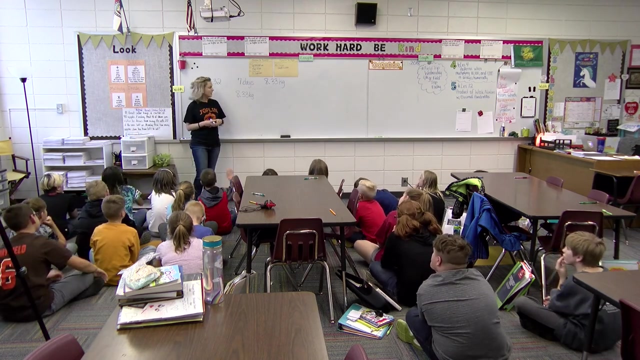 Chloe: Eight and thirty-three hundred kilograms. Now, how many days did we say they're going to be gone? Kaylee: Seven, Seven. I want to draw something to help organize my information, So I'm going to draw what they call the tape diagram, if you guys remember. 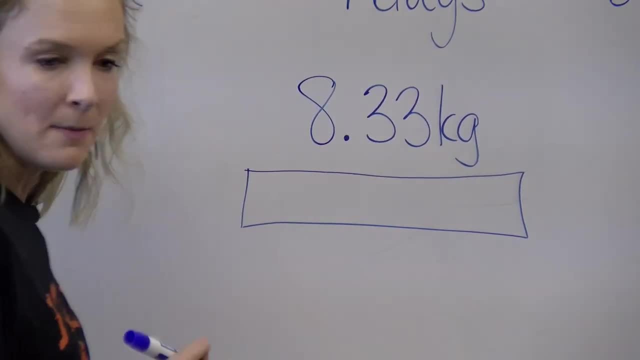 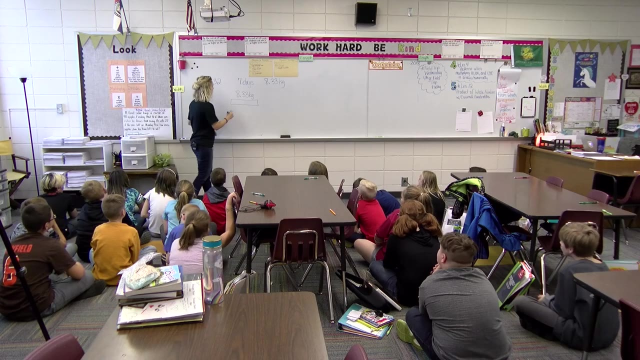 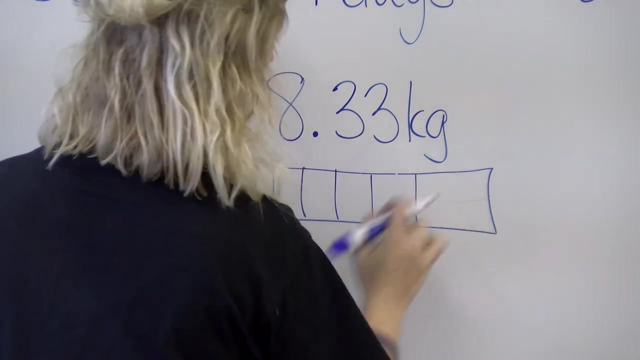 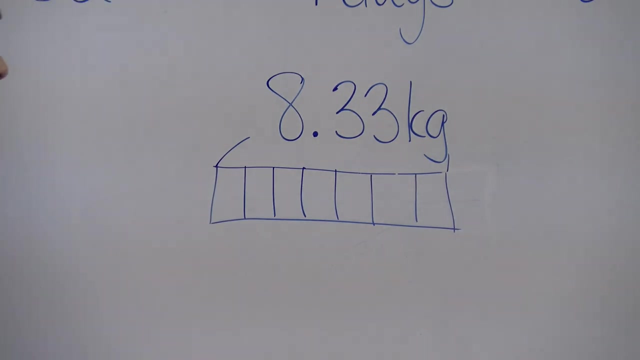 And I'm going to break it into seven parts. Why am I breaking it into seven parts, Alexis, Seven days, Oh, seven days, Okay, I was just checking. Okay, So we're saying, across seven days, each cyclist will require eight and thirty-three hundredths. 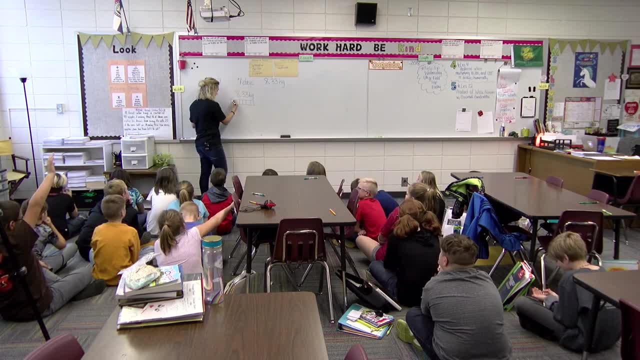 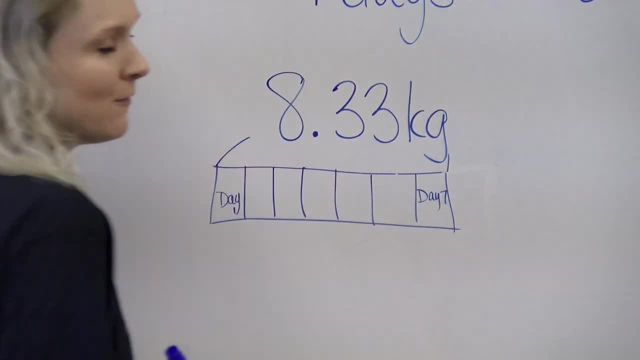 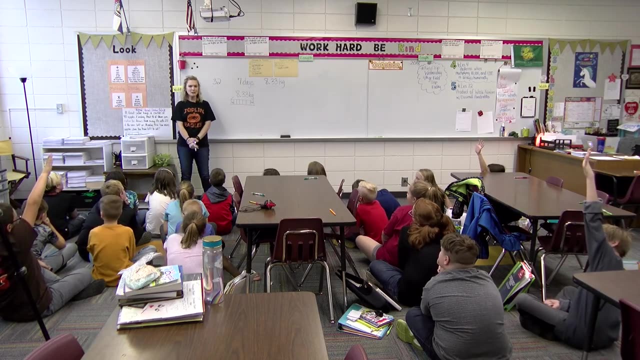 kilograms of food. Okay, So each of these boxes represent a day, So day one all the way through day seven. Here's my question for the team: Do we know how much food each cyclist will require per day? Do we know that? 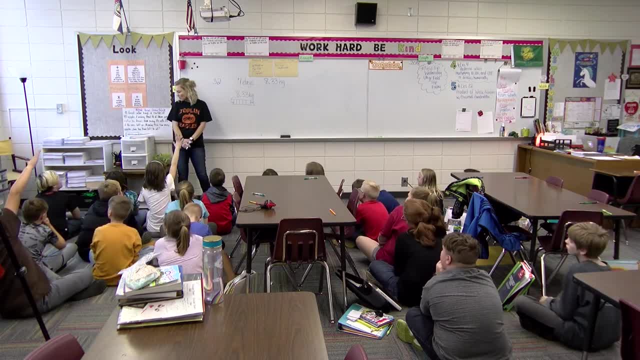 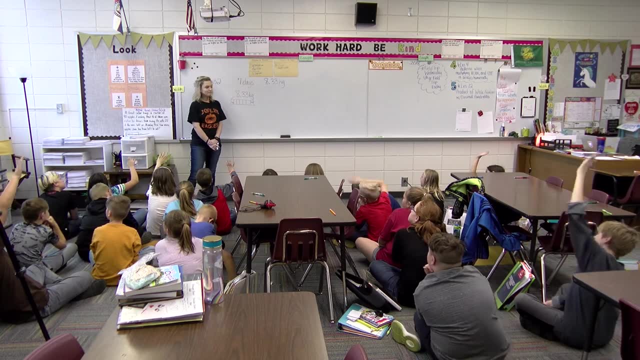 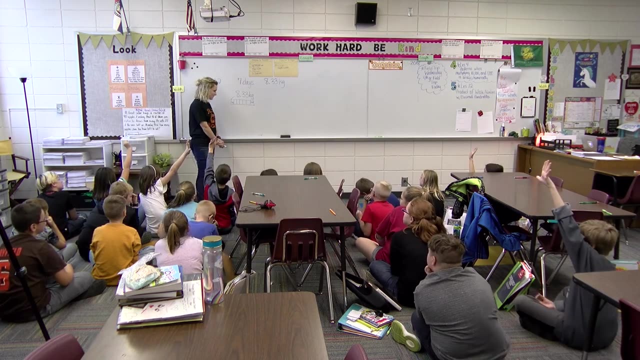 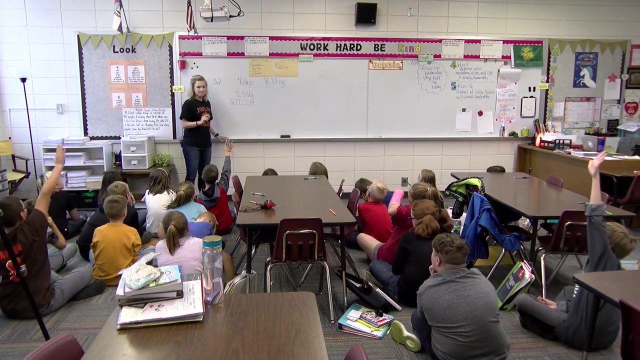 No, No. So someone tell me how are we going to solve for how much food they require per day, Cooper? Not quite Good, try. Appreciate the efforts, Elena. I wouldn't multiply because this is our whole. This is what we're working with. 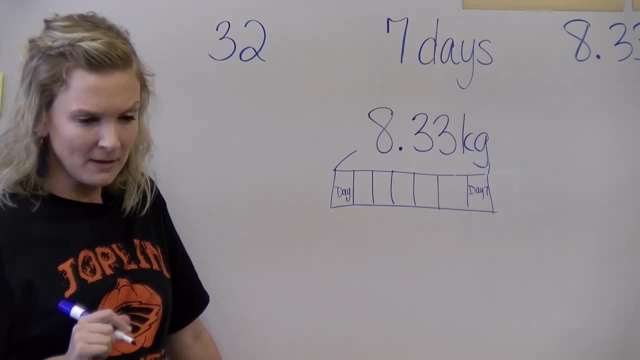 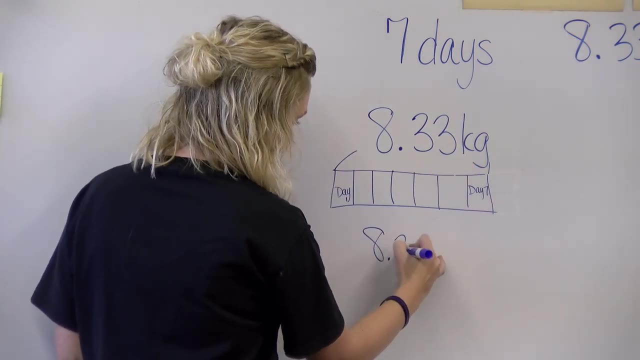 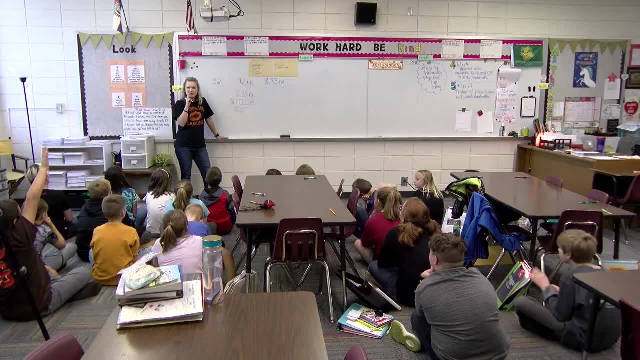 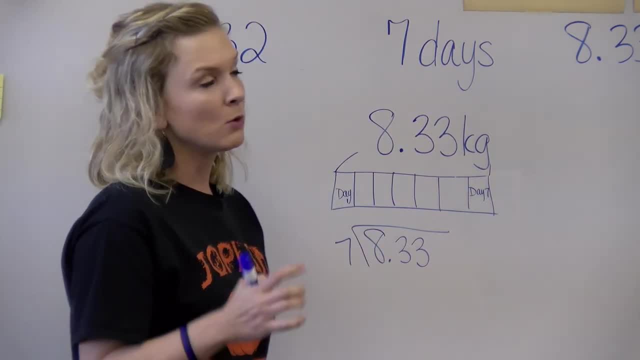 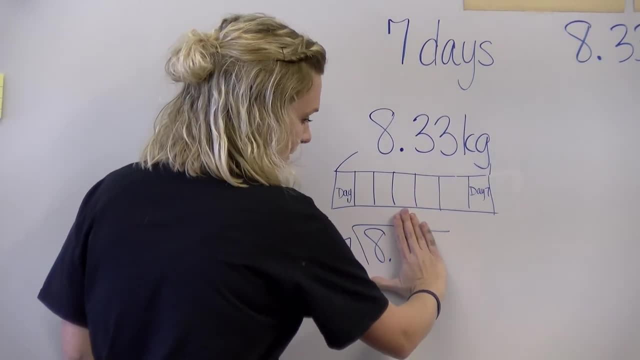 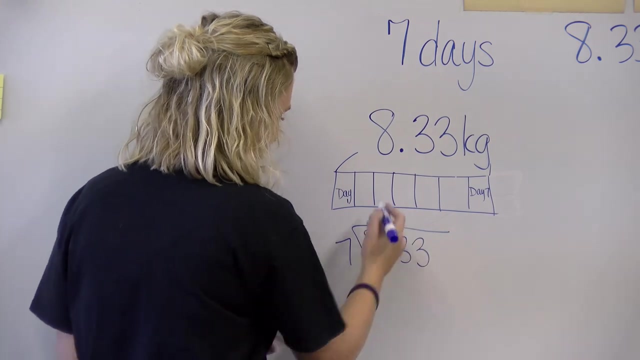 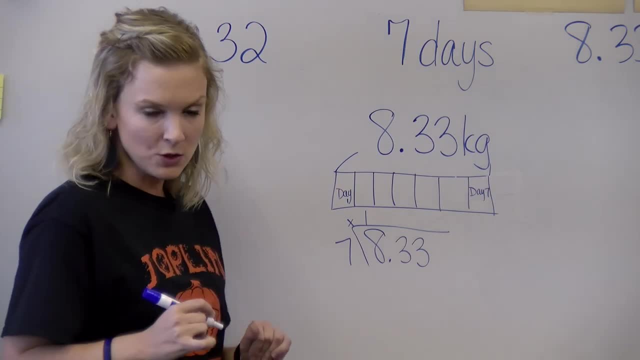 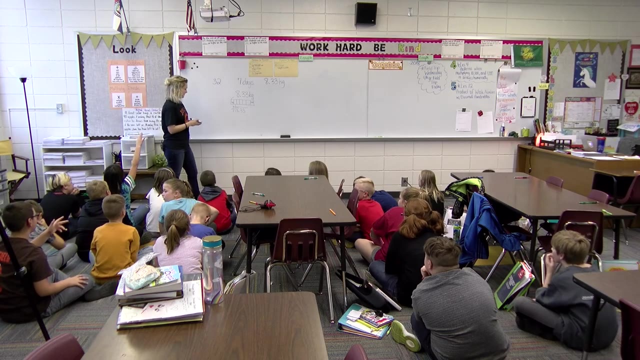 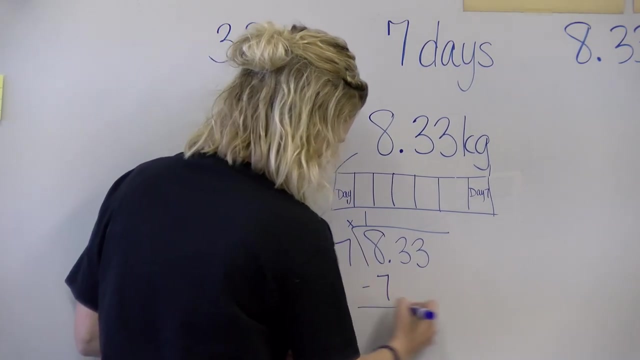 One, One, One, One, One, One One. Why 1 is 7 times 1 is 7, and 8 minus 7 is 1.. Okay, thank you. Bring down the 3.. Now I need someone else to help. 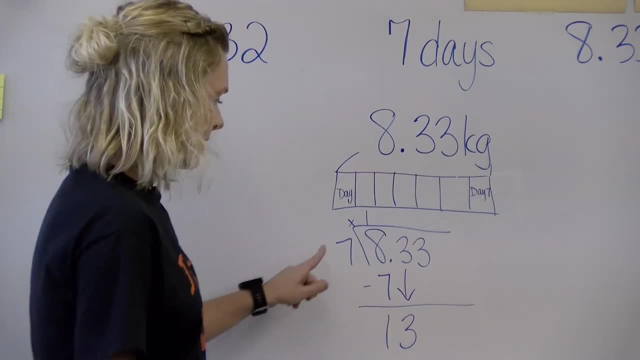 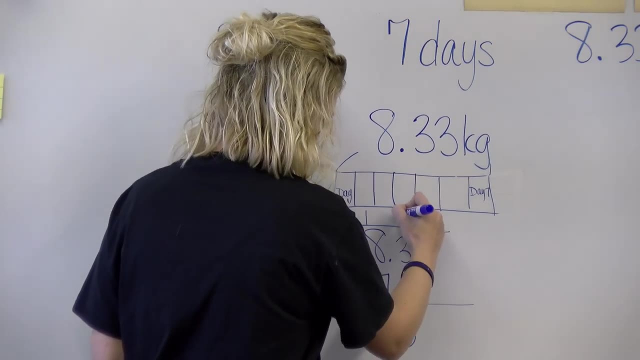 He started us out for the next round. So now we're going to say: how many times will 7 go into 13?? Cooper, One time, because we can't go over right. Okay, Cooper, what is 1 times 7?? 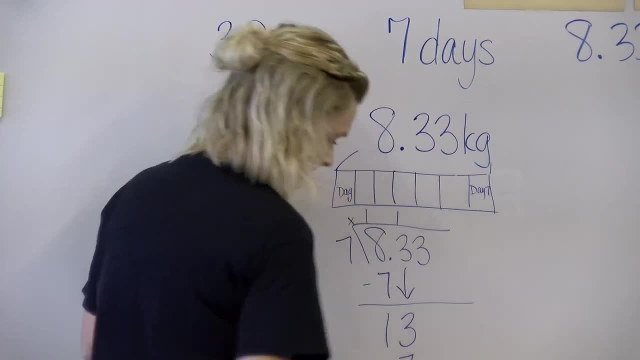 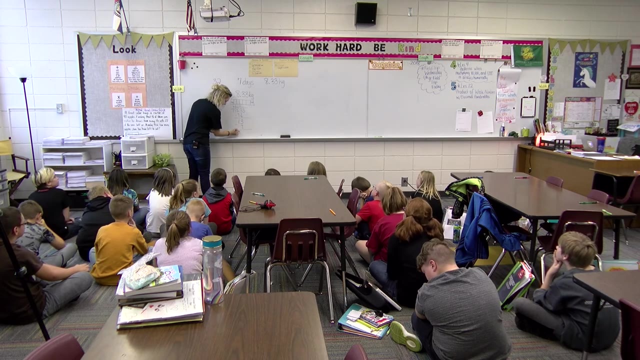 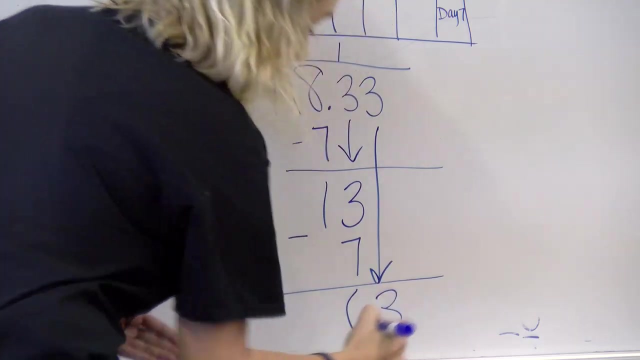 7 minus 13,, which would be 6, bring down the 3.. Okay, so he took 13 minus 7,, he got 6.. Bring down the 3.. Then you're going to start the process over again. 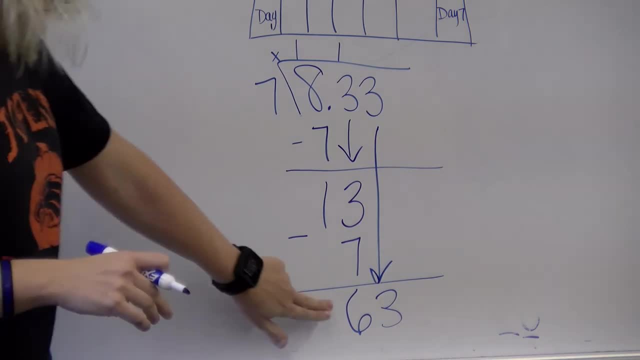 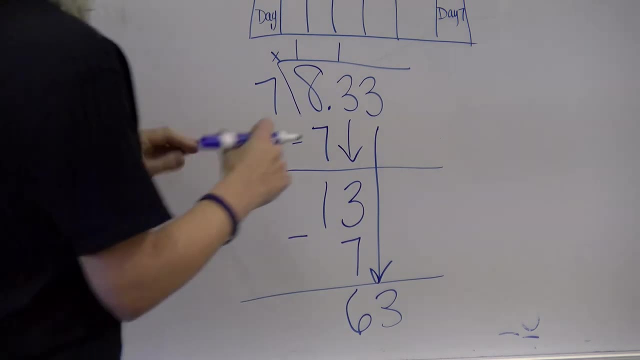 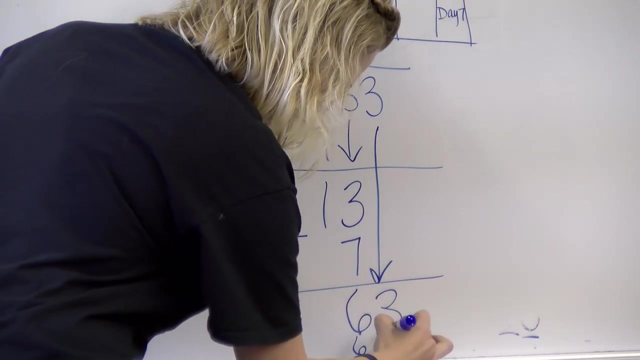 Remember that's part of long division. So now we have 63.. How many times will 7 go into 63? Thomas, 9 times 9.. Thomas, what is 9 times 7?? 9 times 7 is 63, so 63 times 9 is 63, equal. well, 3 times 3, 0. 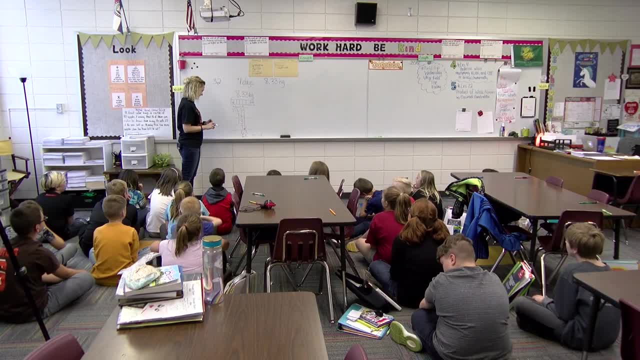 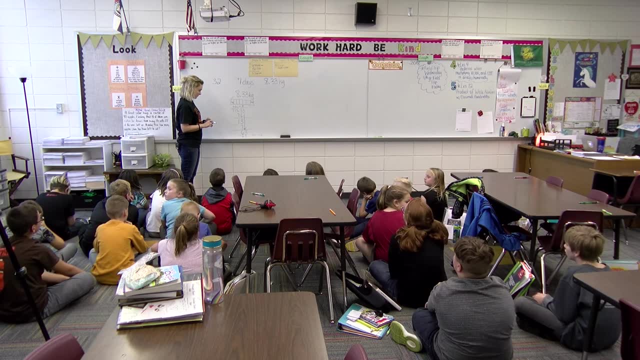 Ran out of space. but yes, 9 times 6 is equal to 0, and I remember when you said: we're dividing, we're using decimals, we're not into the remainder yet, so we have no remainder. Okay, you mentioned the decimal. 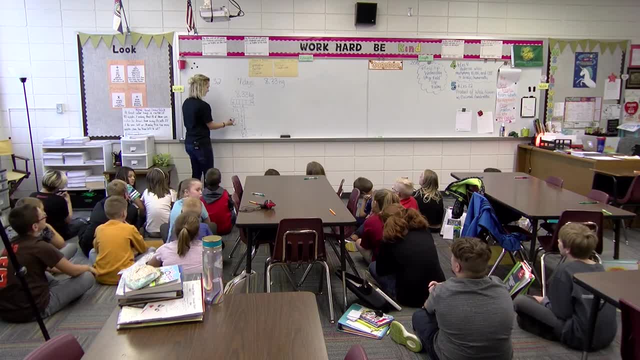 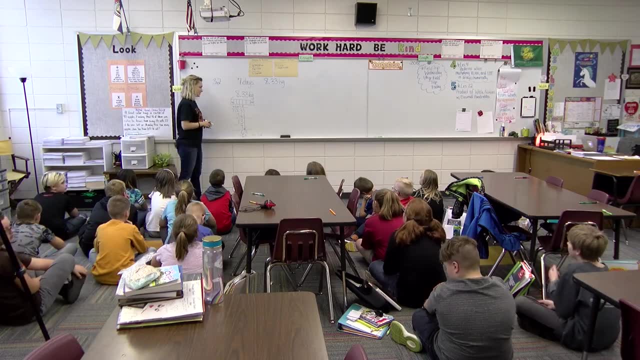 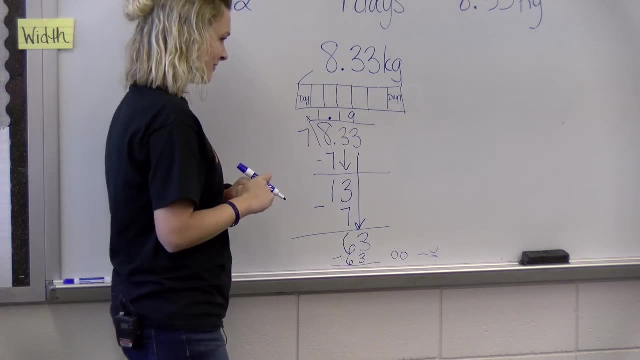 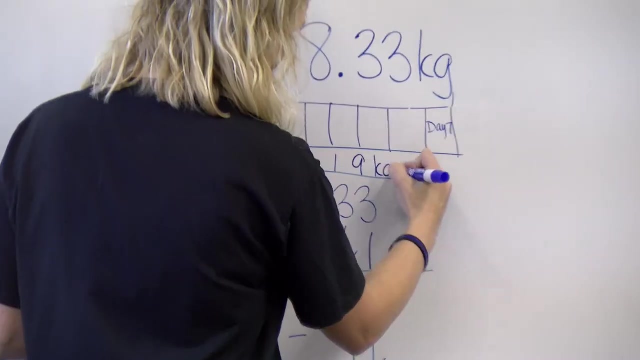 Do I have the decimal in my answer? No, but the decimal goes in between the zero. Nope, it goes right here. Someone tell me what did we just figure out, Elena? How much food they require for each day, How much they require per day, which is 1 and 19 hundredths kilogram worth of food. 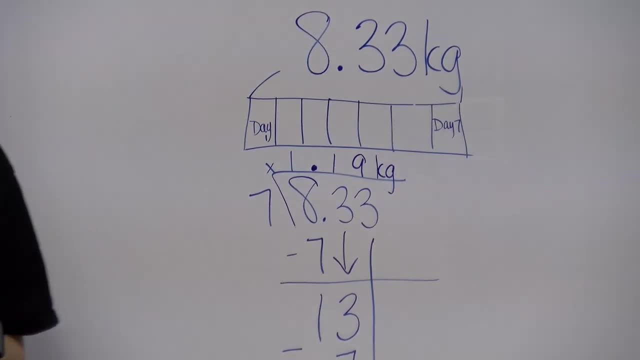 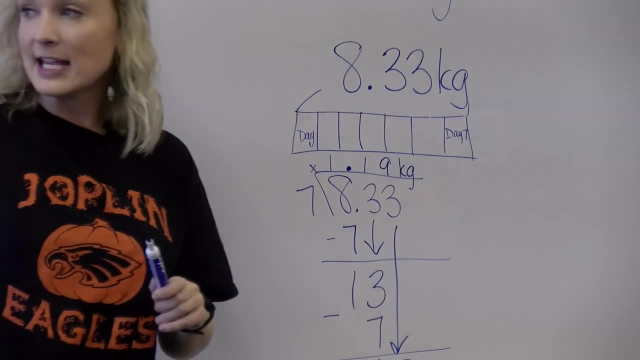 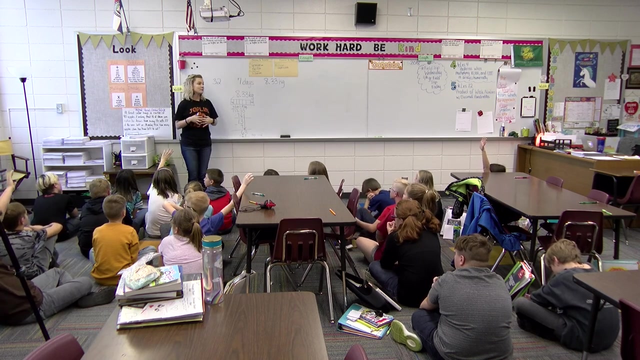 We're not done yet. Okay, question, Okay, hold on. Now. step two: listen in Day five, correct? They said: how much are we carrying at the end of day five? How many days would we have left on our trip if we just ended day five? 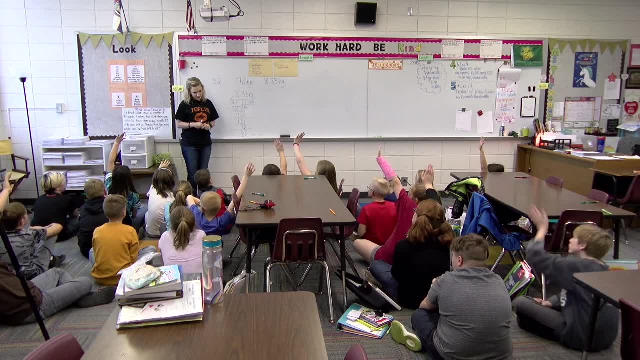 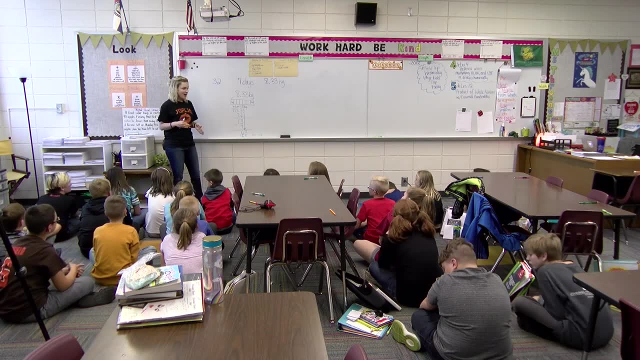 We just ended day five. How many days do we have left for our trip? Evan, Two Two. So we've ended day five. Now we need to figure out how much food will be required for two days. You follow me so far. 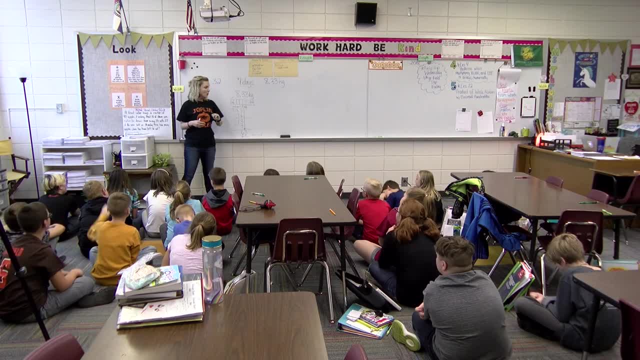 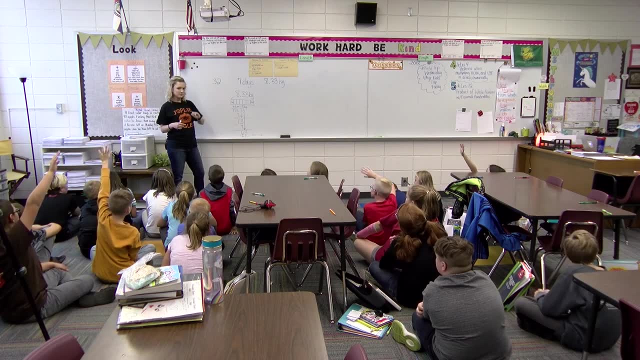 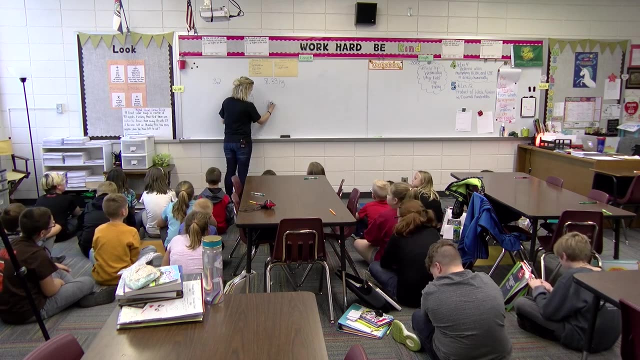 Day six and day seven. We need to think about day six and seven. So what are we going to do with our per day amount in day six and day seven? Cool, I would agree. Who would like to help with the multiplication? 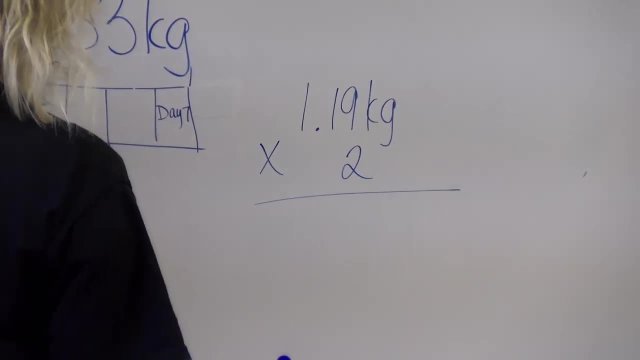 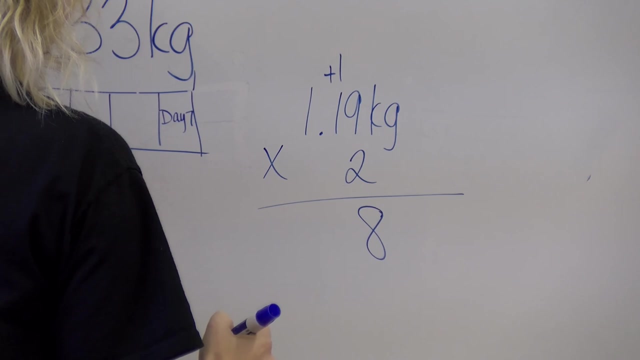 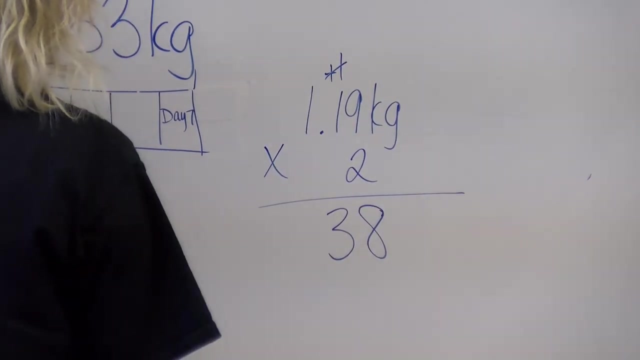 Alexis, Two times nine, Eighteen, Eighteen, You put this together: Two times one, Three. Two plus the one is three. Yes, ma'am, You're good, Cross out the one, Okay, Two times one, Two. 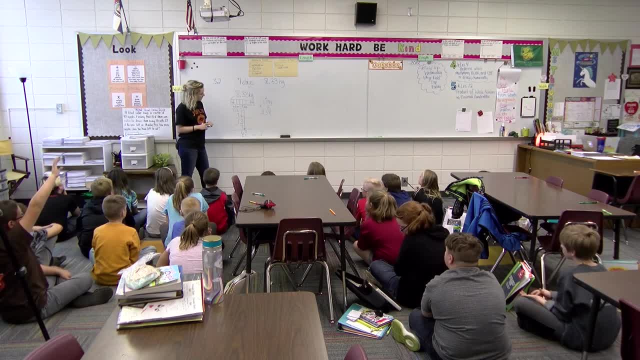 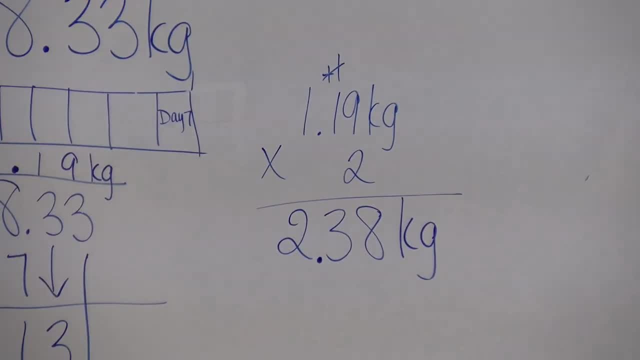 Alexis, where is my decimal going to go in my answer? In between the two and the three, The two and the three? Someone tell me what did we just find with two and thirty-eight hundredths kilograms? What did we just find here? 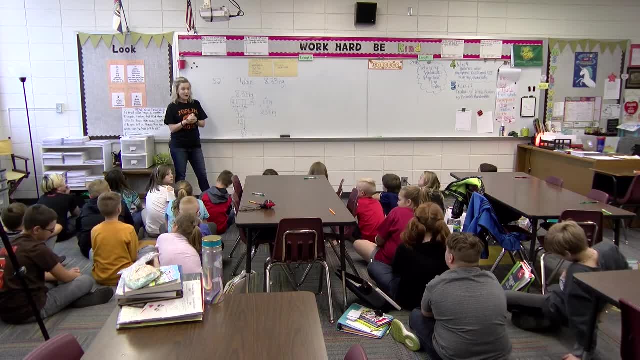 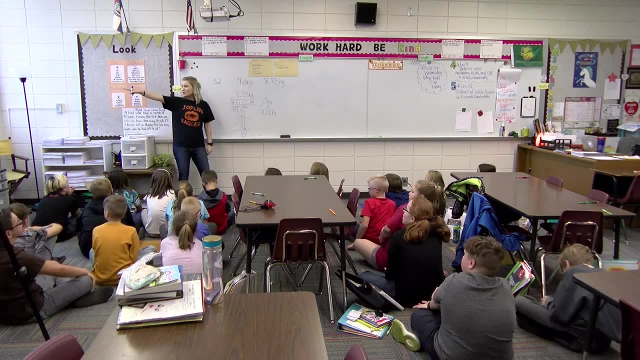 Cole How much food they're going to need for those remaining two days of the trip. right, And that's day six and day seven. But they threw us an extra little something and they said: how much food will the group carry? 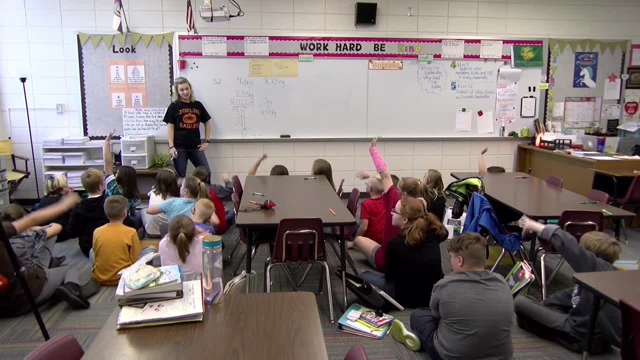 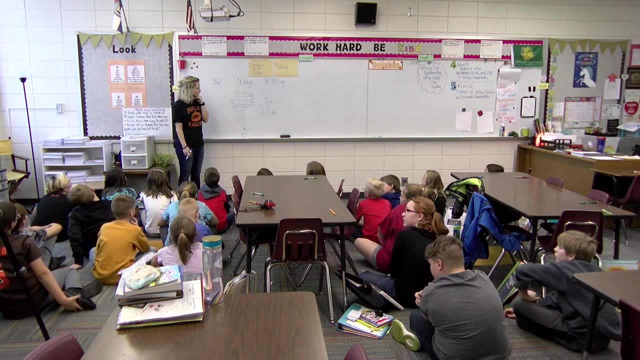 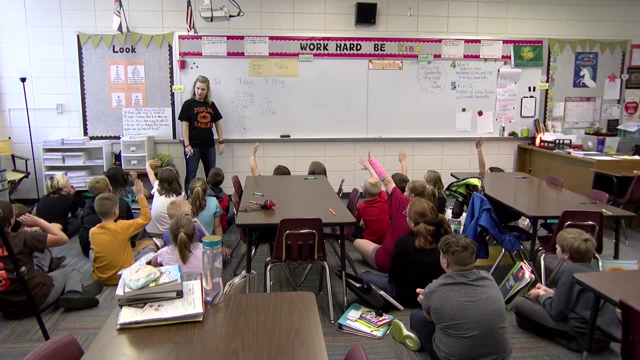 Well, how many people are in our group, Charles? Thirty-two. Thirty-two people, Thirty-two people. So what are we going to do with that thirty-two the group and the amount of food needed for day six and day seven? 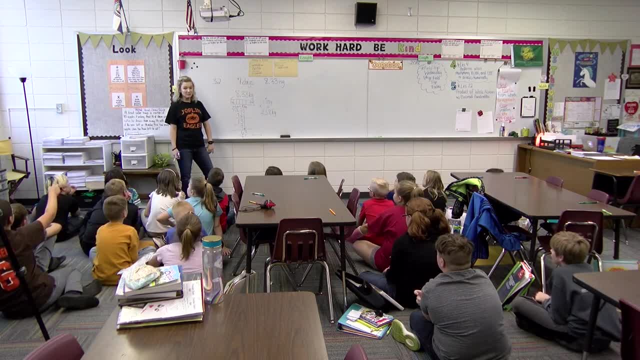 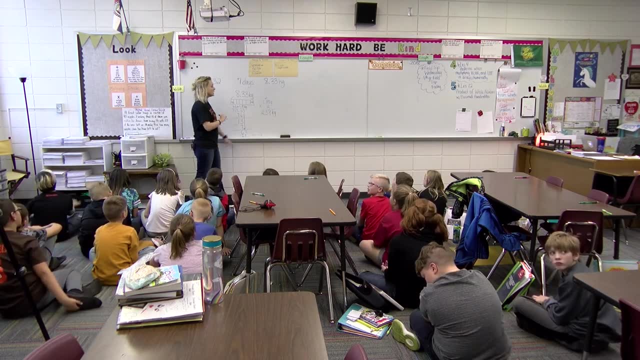 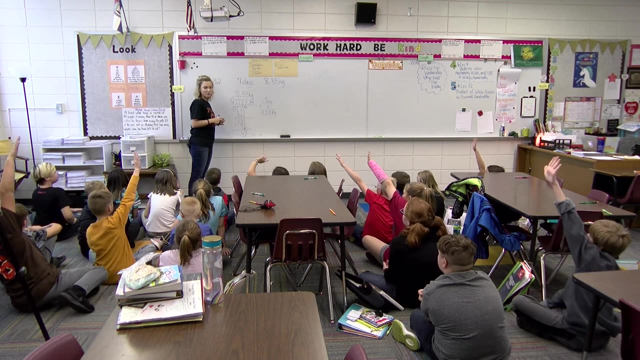 I would agree. No, I would times it. Man, that's a lot of food. No, you're good, I agree with you. So question: Could I rename this over here when I set up my multiplication, Could I rename that into my unit form? 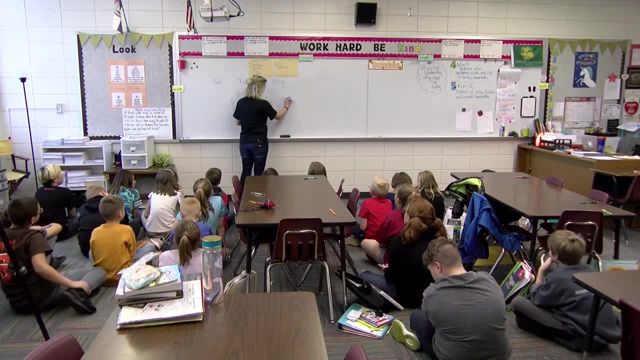 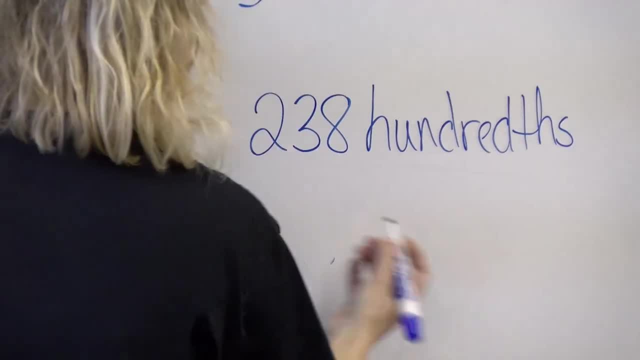 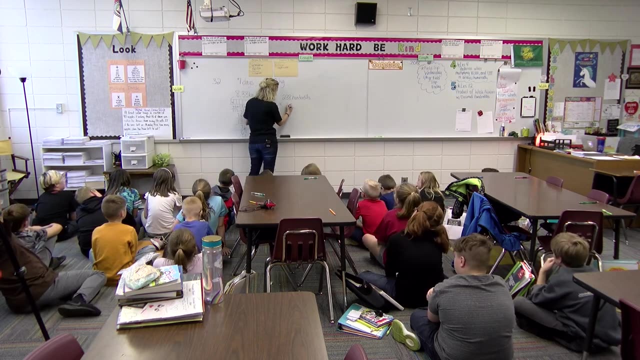 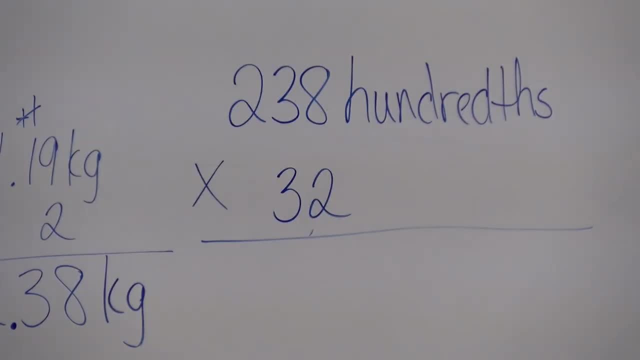 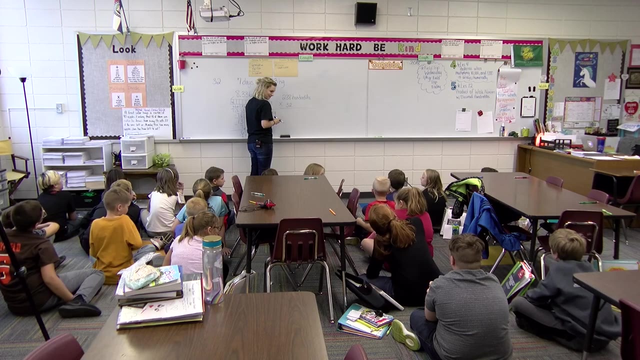 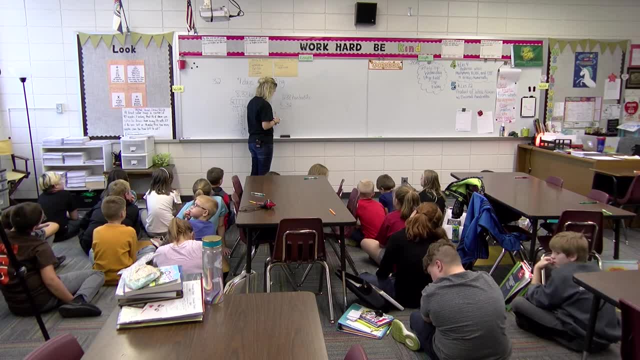 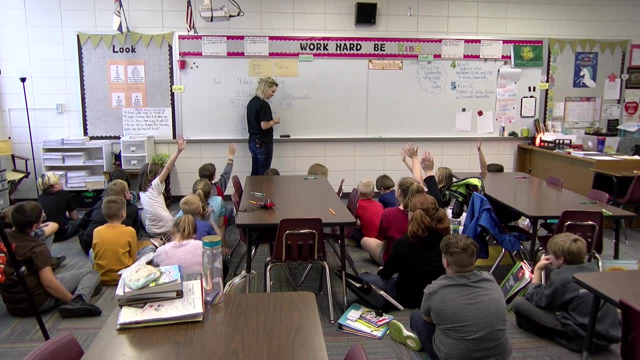 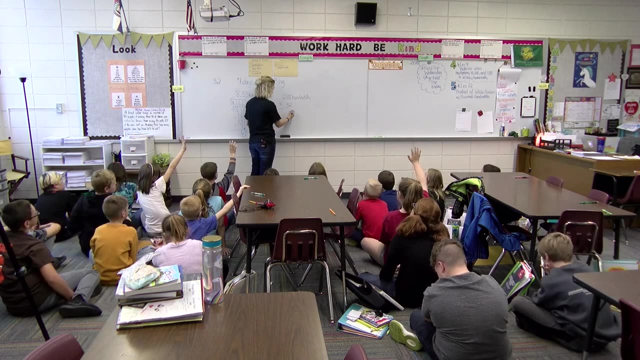 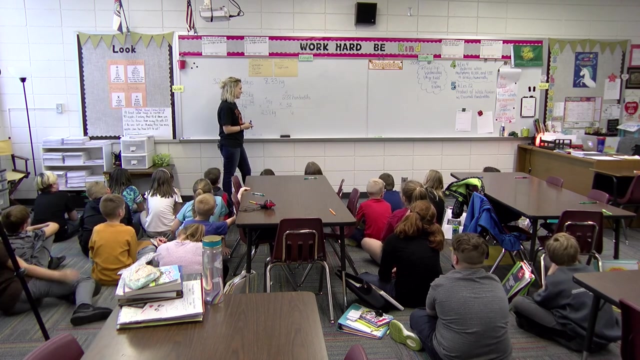 Multiplicate, Multiplicate. Not quite. I appreciate your efforts, Jade, Sixteen, Sixteen. You're going to put the six down. Carry the one Two times three. Elena, Six Plus one. Thank you, Kaylee, two times two. 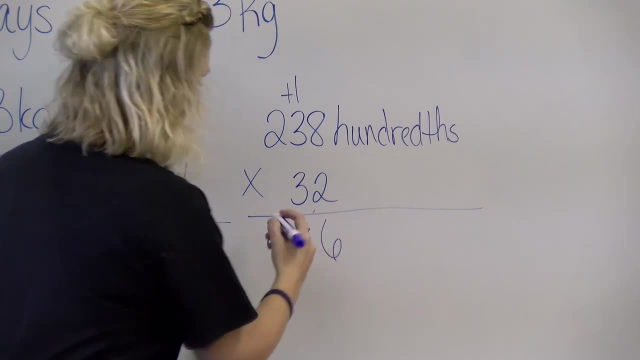 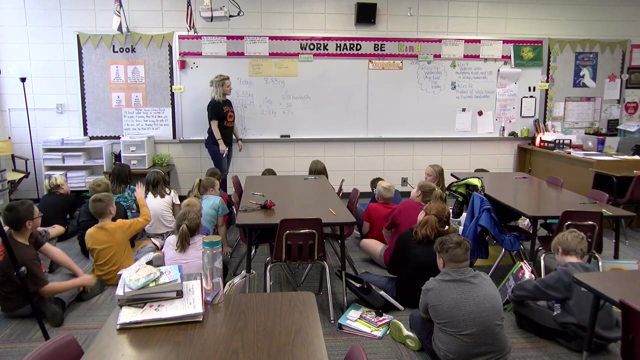 Four, Four. Okay, Someone tell me We're about to go into something very important. If we don't do this step, we might mess up our answer. What is it, Cooper? We're going to cross out the plus one and the ten and put a zero under the six. 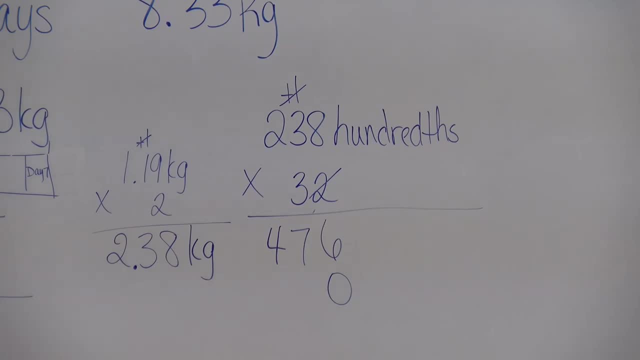 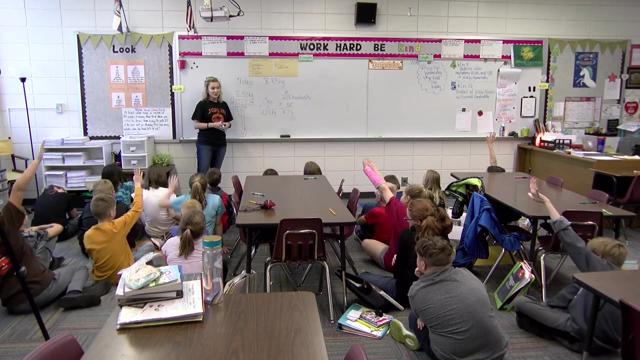 Why would I need that zero? What does it tell me I've done? It tells you that you're done with the ones place. I'm done with the ones place, So now I can go into what place value Kaylee, The tens place. 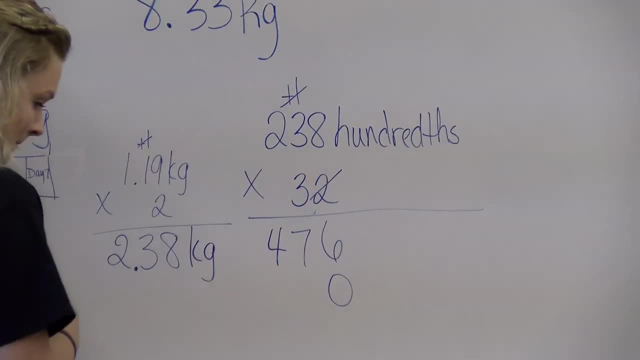 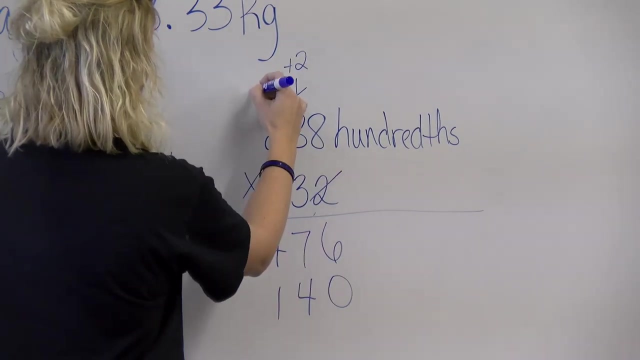 Ava, what's three times eight, Four, Four. Okay, So I'm going to put the four down and carry the Two. Ava, three times three, Nine Plus two, Eleven. You're going to put the one down and carry the other one. 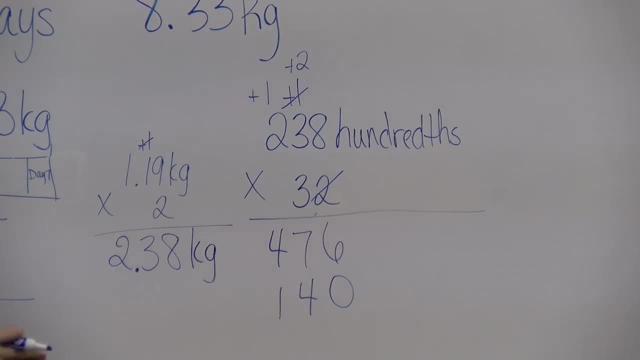 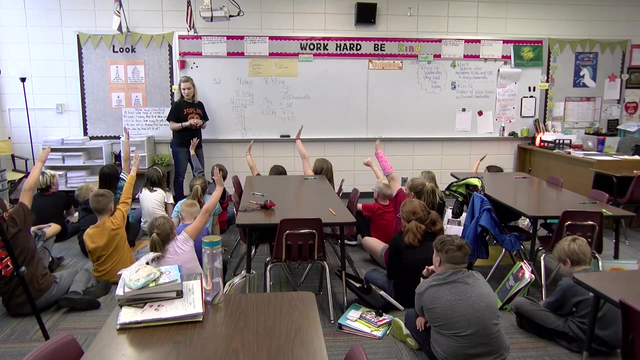 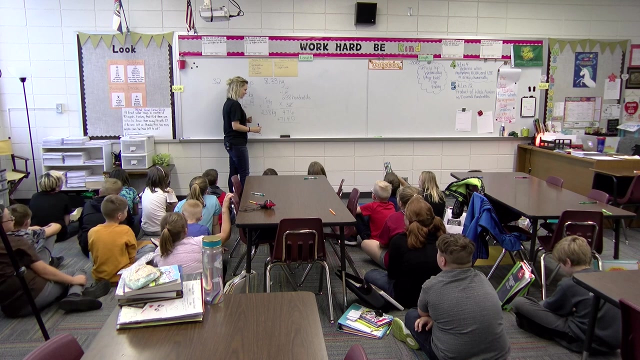 Three times two, Ava. Six Plus one is seven. Yes, Thank you, Ava. Someone tell me What's that final step? to finish out my standard algorithm of multiplication: Olivia: Add, Add, Add, Add. It's Finished. 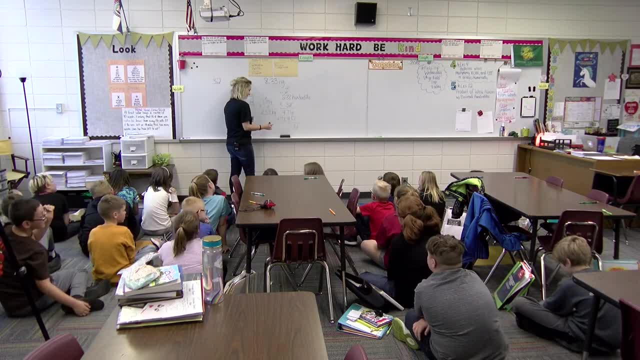 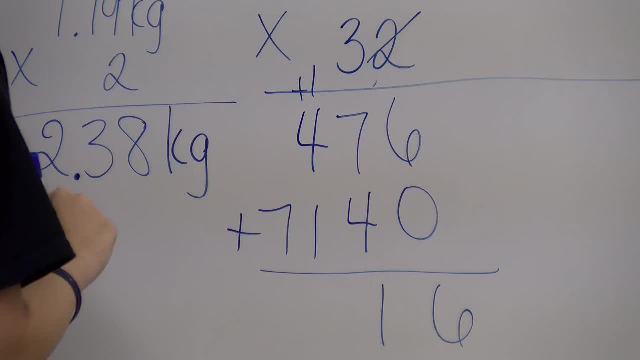 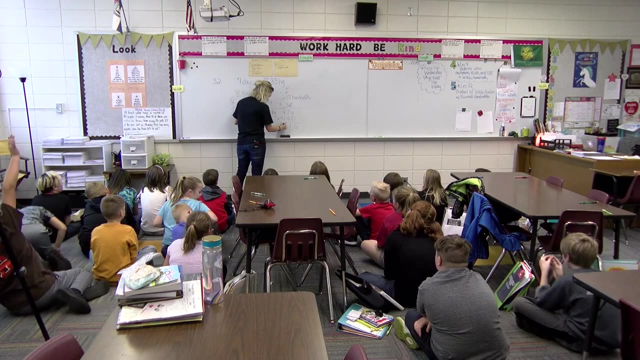 One. I got it done. All right, Olivia, Here we go. Six Plus zero, Seven plus zero, Seven plus four, 11. Put the one down and carry the other. one. One plus four plus one, Six, Seven plus nothing. 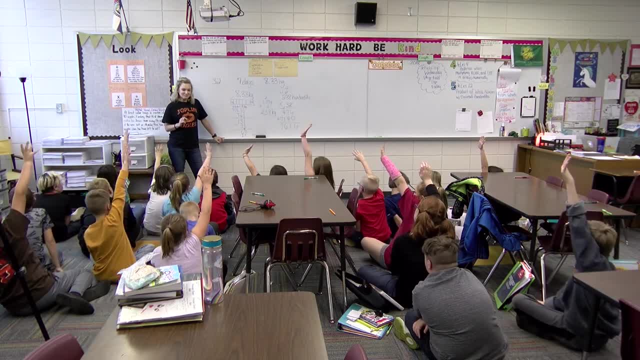 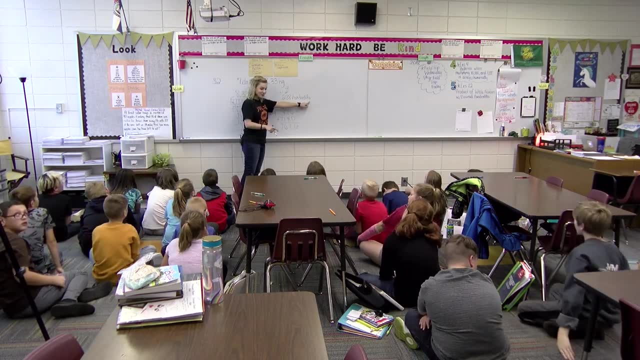 Two Now question from my team: What am I missing? What am I missing, Megan? My decimal, because when I renamed it it told me my place value, that I needed to focus back in with that decimal. Where's that decimal going to go, my friends? 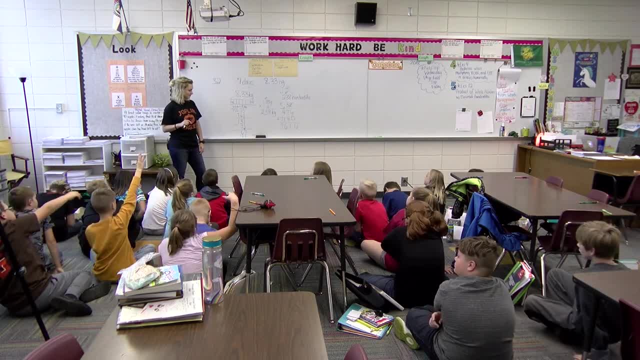 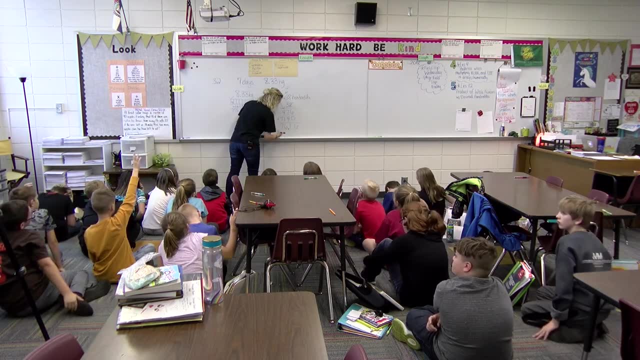 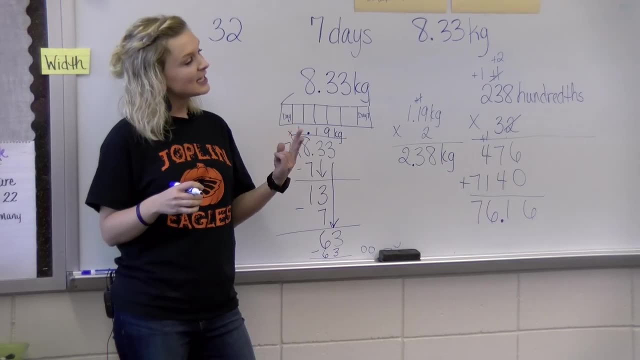 Charles, The decimal's going to go between the six and the one, Which, Ooh good, catch buddy. So someone tell me how much food is the team going to carry for day six and day seven of our trip, Alexis? 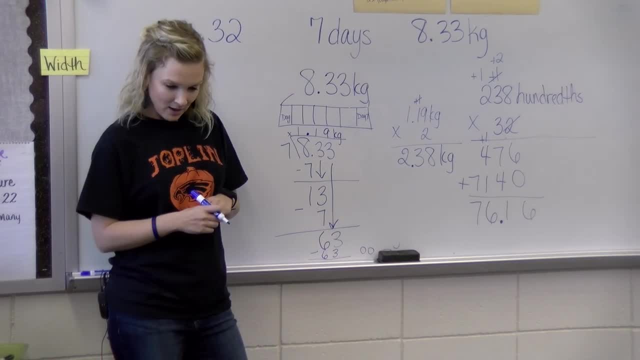 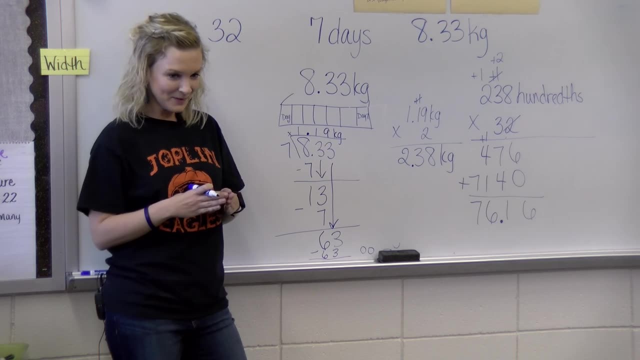 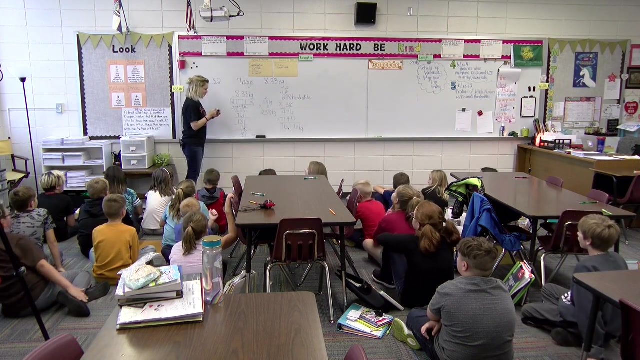 Seventy-six decimal point. sixteen hundred Seventy-six and sixteen hundred. Yes, ma'am Cole, I forgot something: You have to put kilograms. I do need that label, because we're talking about our weight of food. Now, What do you guys notice with the work we had to do here? 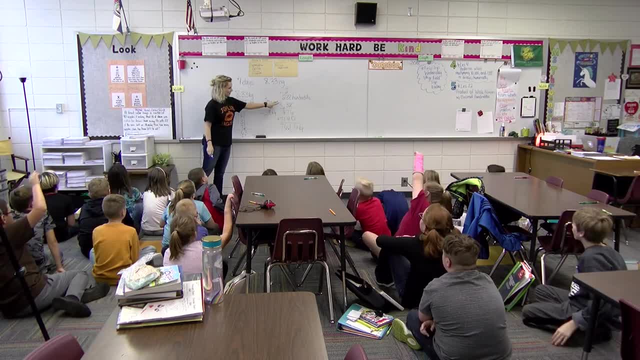 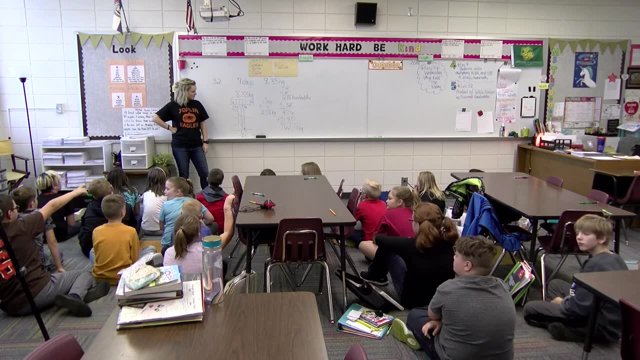 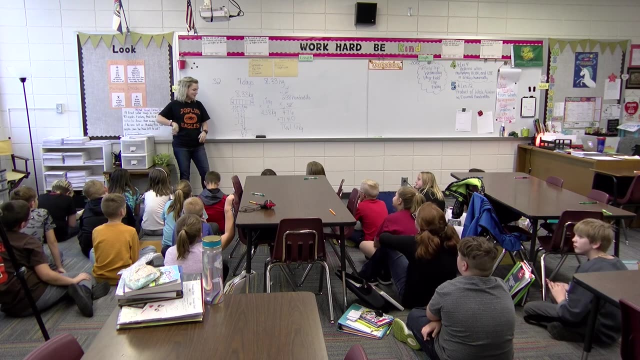 How many steps did we do? Two, Three, Three, Three steps to answer one question. Way to go, friends. Yes, sir, It actually beat four, because you added it too. Yes, Now, very good job. That could have been really tricky, but you guys did a fabulous job with that. 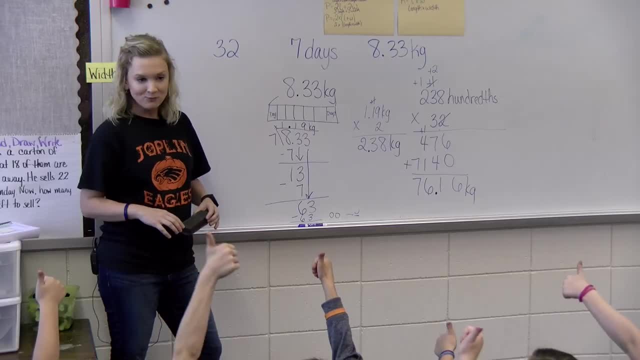 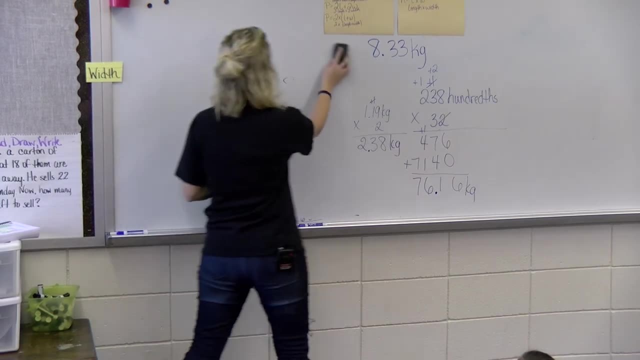 Give me a thumbs up if you are ready to go into our lesson. All right, friends, here we go. I appreciate what I'm seeing with our efforts. Let's continue. Now we're going to quickly review what we've been doing. 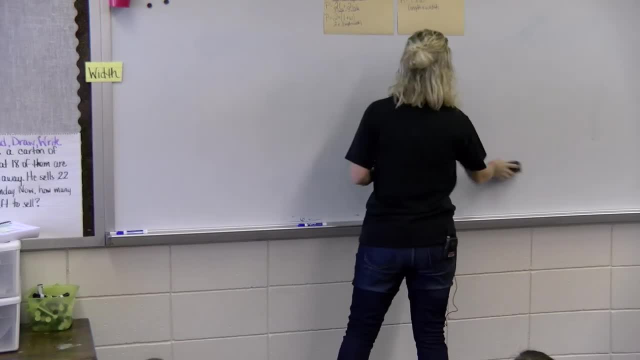 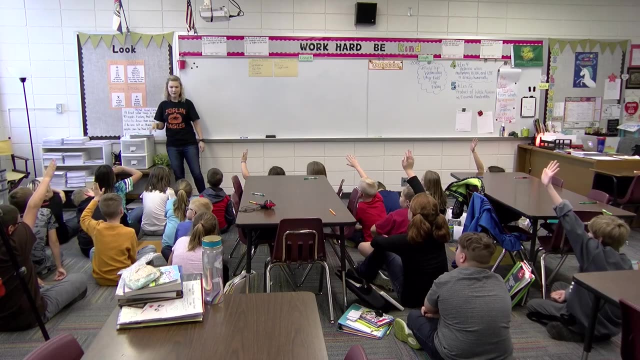 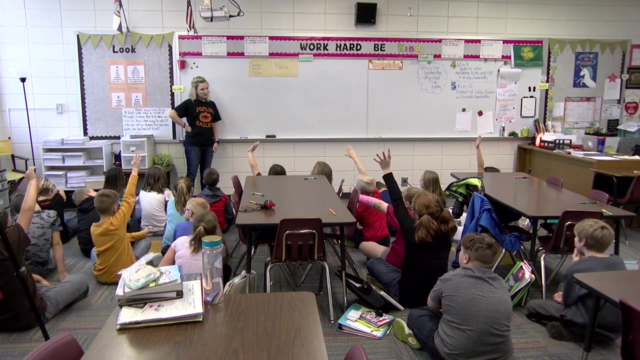 which is estimating our factors to get the estimated product. Then we're going to do the standard algorithm. Can someone remind us what is standard algorithm? That's a big word, London, Not quite. You're on the track, Kaylee. 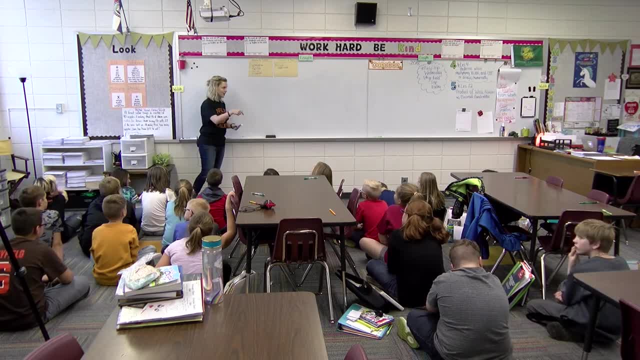 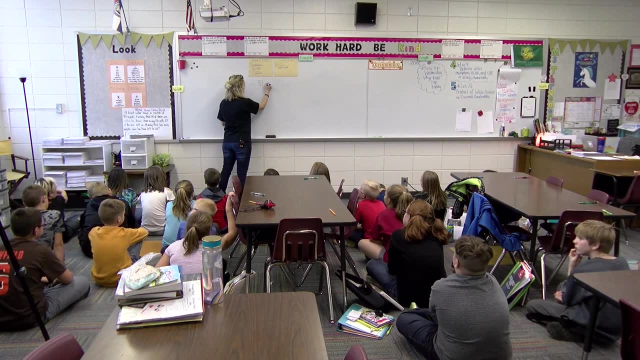 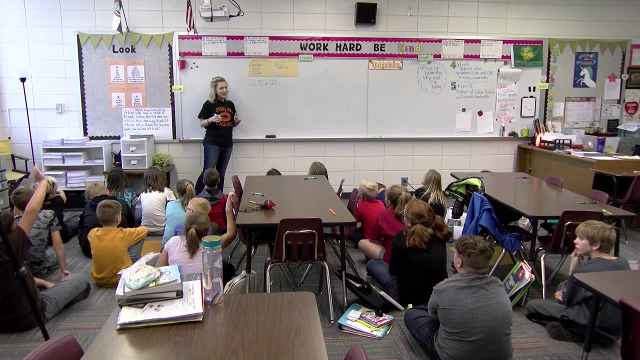 Just the standard problem. Okay, Those big words, they're not going to get us. So here's our problem. Two and thirty-one hundredths times twenty-two. Those are our two factors. I need someone to help me estimate two and thirty-one hundredths to the nearest whole number. 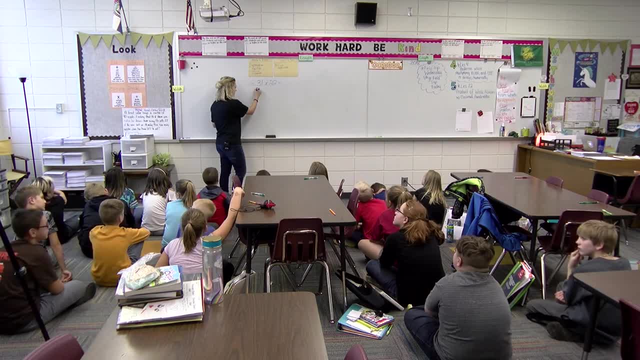 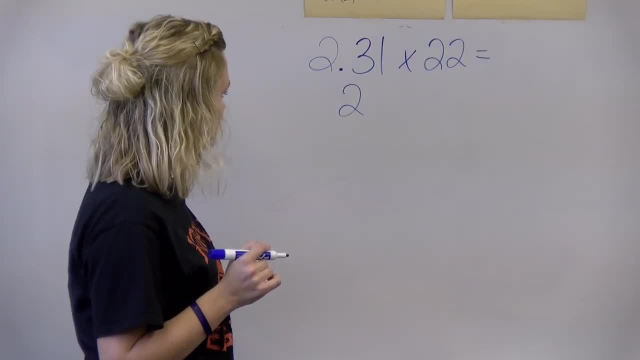 Ethan: Two, Two. Okay, Ethan, how did you know it was two? Because you looked mainly at only a focus on the times. twice Okay, so you looked here Because at hundreds of places you don't have to focus on it. 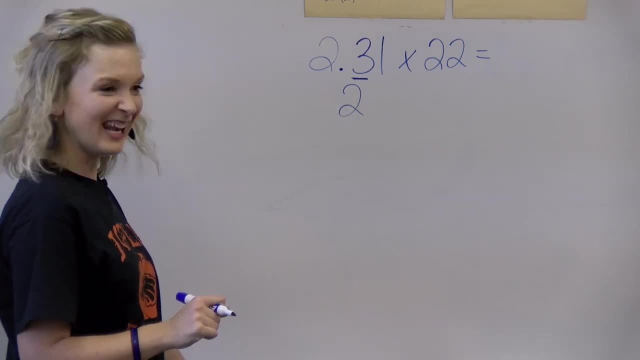 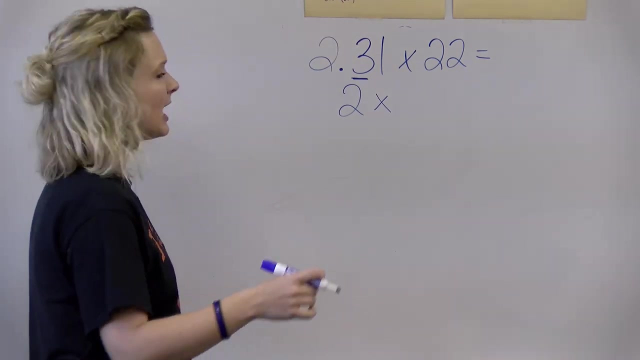 That's just dot work that you don't actually do, And so if you know how to estimate, you know that if it's twelve-five you can estimate to the lowest number. I would agree. I love the explanation. Thank you. 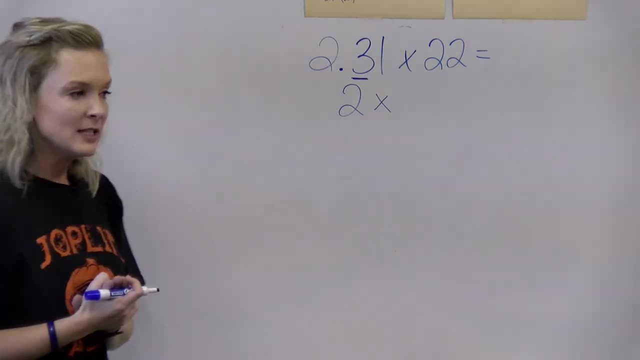 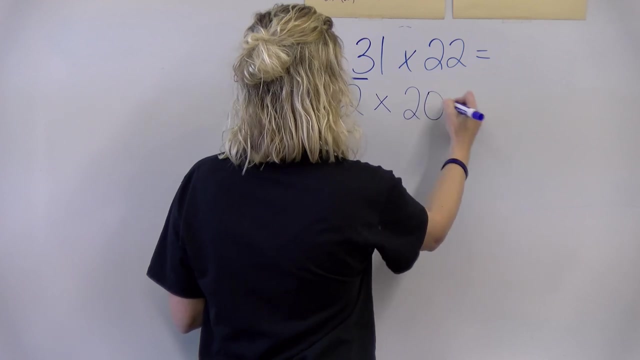 Now twenty-two. We need to round that to the nearest tens place. What would we estimate it to, Chloe? Twenty, Twenty, Twenty. So, using our estimated factors, can someone tell me what is my estimated product? Olivia? 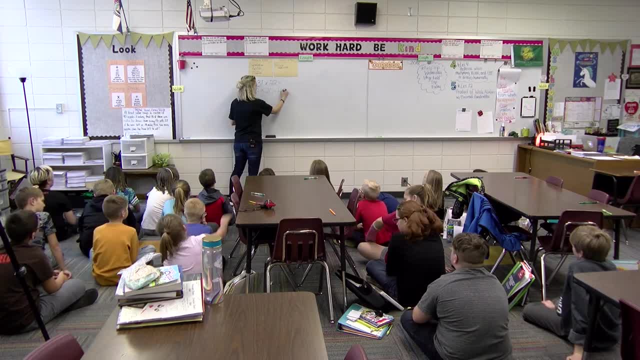 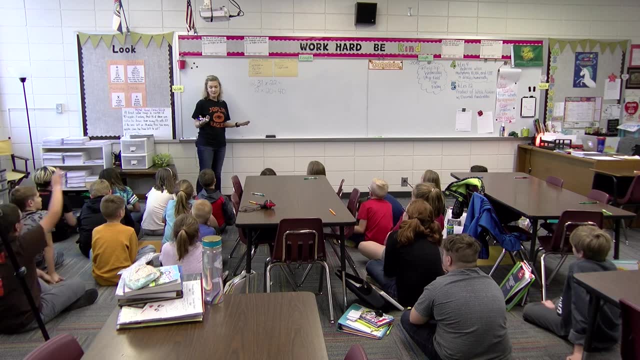 Forty, Forty. How did you get forty, Olivia? Because you just take out the zero and you do two times two and then you just add back in the zero. So you focused on the basic fact. Oh, that was awesome. 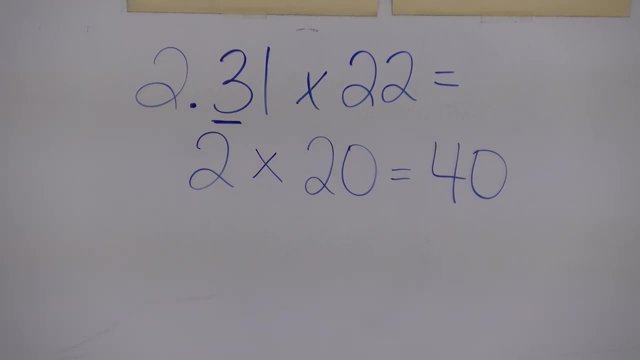 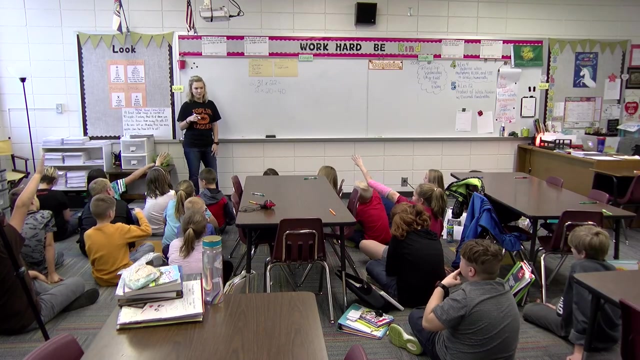 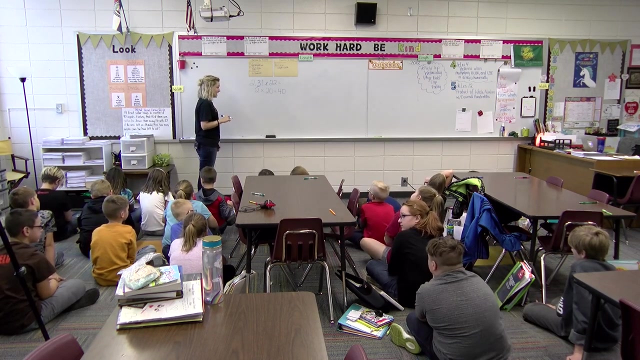 Now we're not done yet. We now have to do the standard algorithm, which Kaylee said was the standard problem. What factors are we going to use for the standard algorithm? Cooper, Two, Two and thirty-one-hundredths and twenty-two. 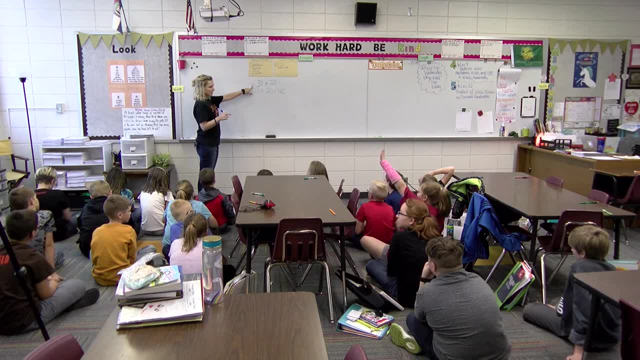 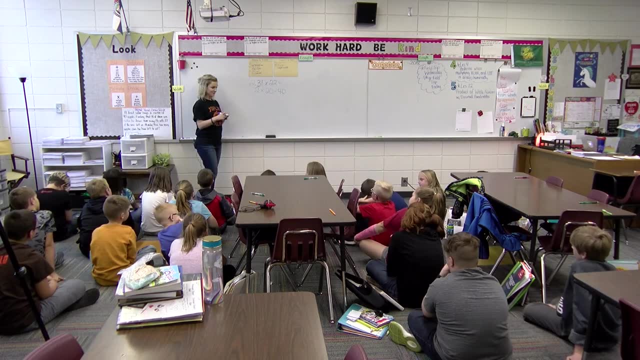 Now, Cooper, you're correct, but what do you notice about this factor right here? That we need to rename it into two hundred and thirty-one-hundredths? I would agree, Cooper. why do we rename it? Why do we take that extra step? 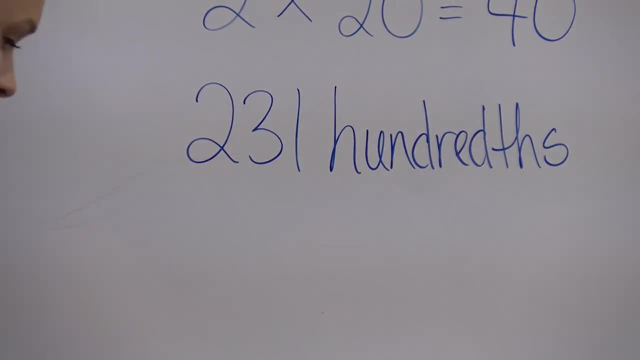 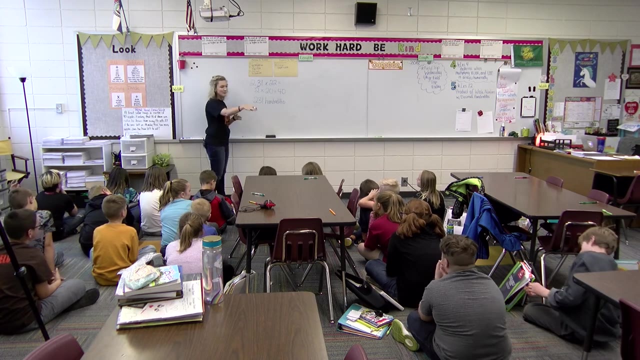 Because it helps you do the multiplication problem- and what color you said earlier- and you don't get distracted. We don't get distracted by the decimal. Now don't we put the decimal in at the end? Yes, we do, But right now we just want to focus on the standard multiplication. 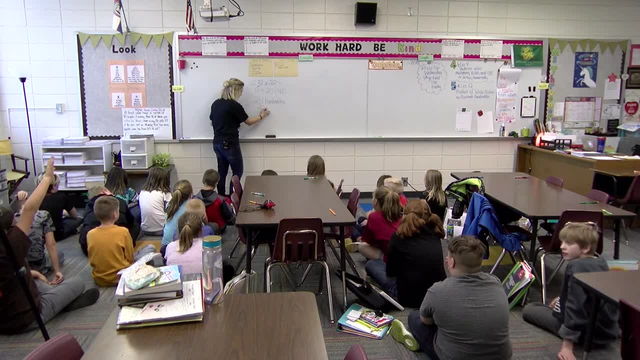 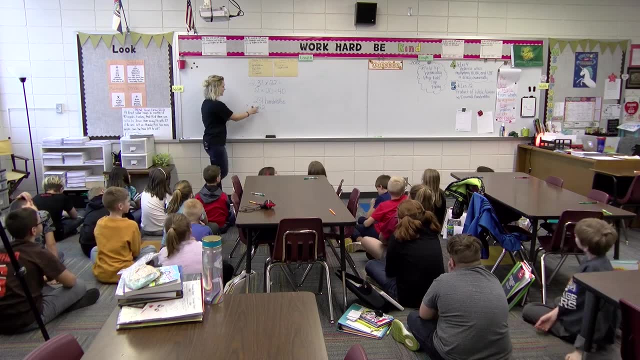 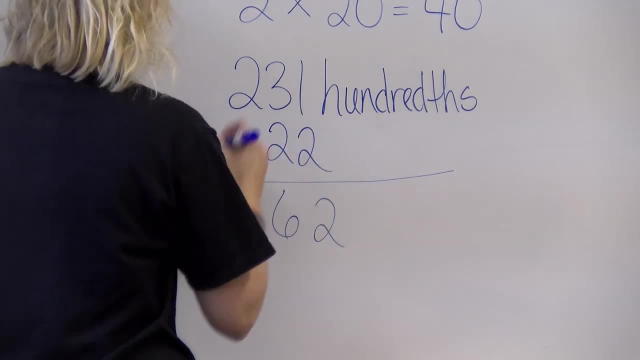 So we're going to multiply that by twenty-two. Who would like to assist me with this problem? Jade, here we go. Two times one, Two, Two times three, Six, Two times two, Four. Now, Jade, this is an important step. 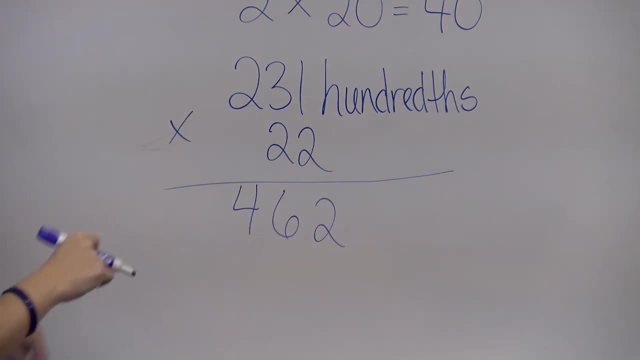 Okay, What do I need to do to get ready for that second row of multiplication? Do you remember Cross out the two? Why would I cross out that two Jade? Because it's in the ones place and aren't we done with the ones? 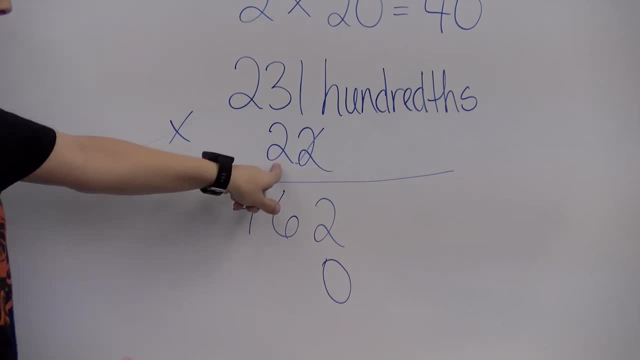 We're done with the ones. now, What place are we going to actually go and work with The tens place? The tens place. I need someone to help me. Who's going to help me, Thomas? I see you Two times one. 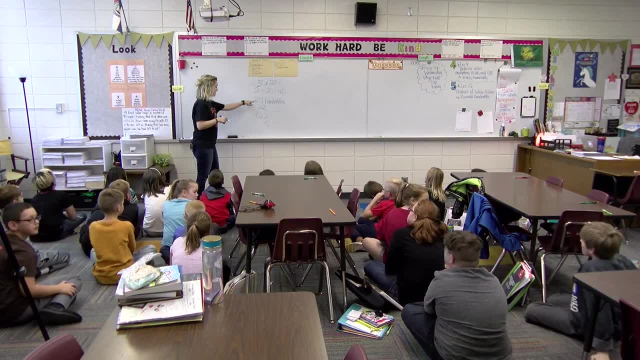 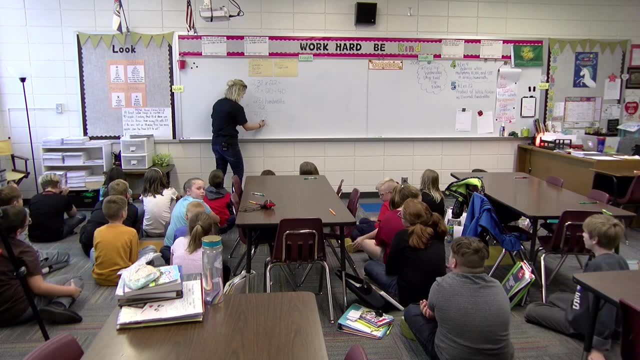 Two times one One. Check again: Two. Okay, Does anything times one equal one or anything Equals itself? I knew what you meant. Two times three, Three times, okay. two times three, Six, Six, Two. 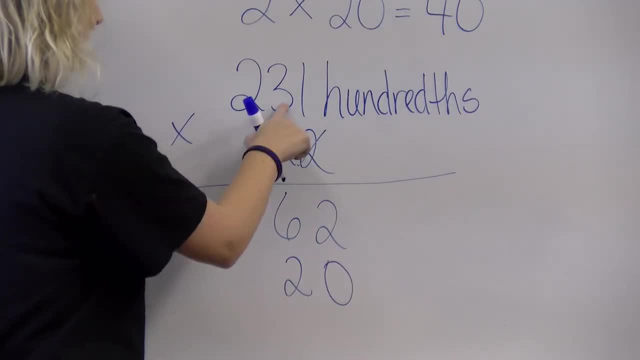 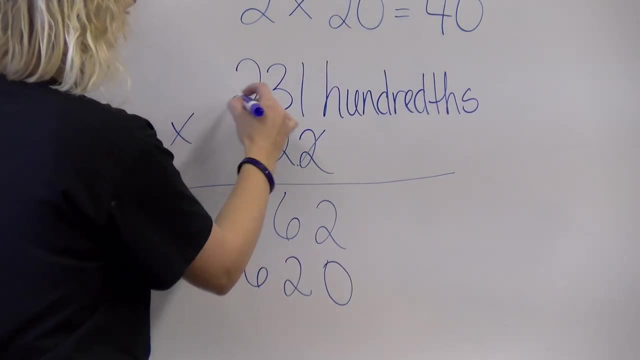 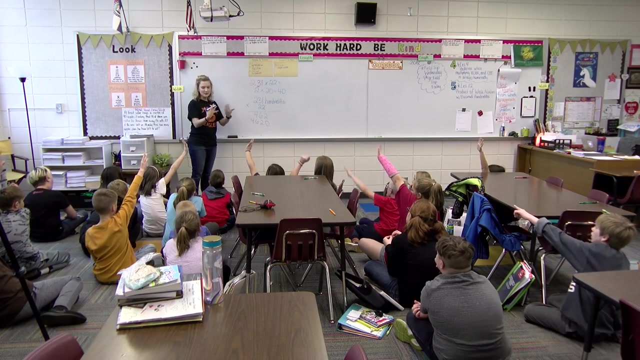 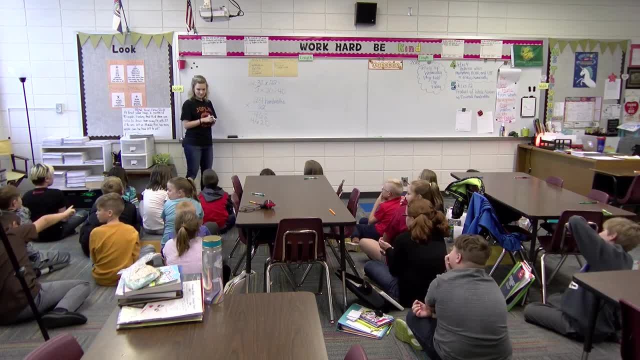 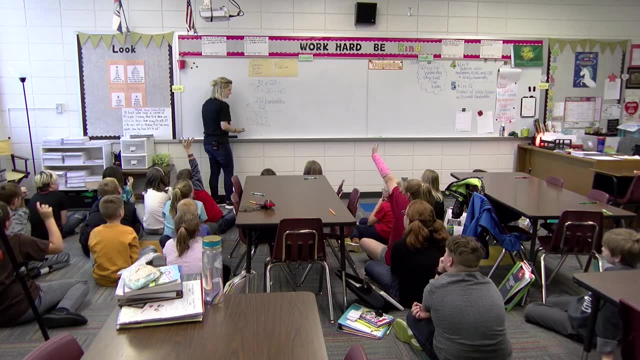 Charles, You're going to add it. Okay, we're going to add up. These are considered the partial products, remember, because they go with the ones place and the tens place Two. Two Because two plus zero is Two. 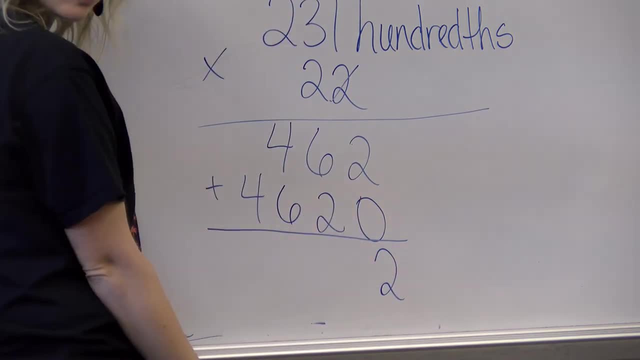 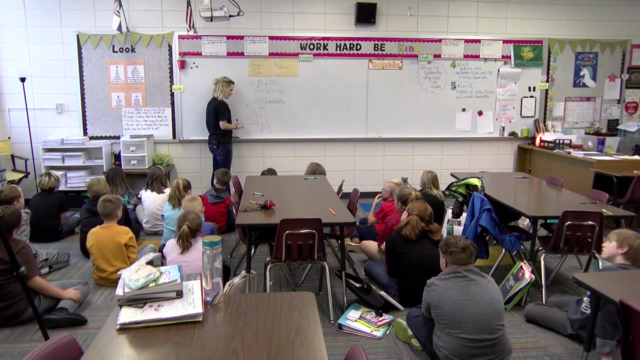 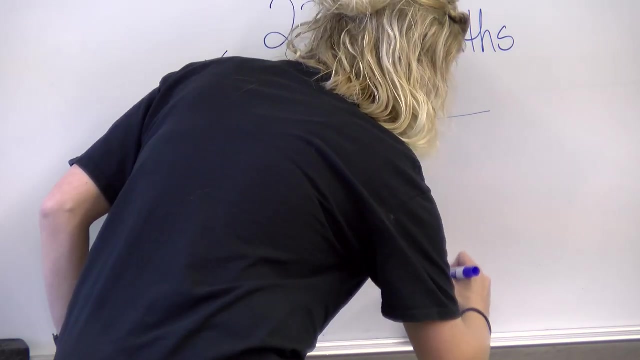 Six plus two. Two Two, Two, Two Eight. Good correction. Four plus six. Four plus six, Ten, Ten, Right, three times one. I like how you used that terminology: One plus four, Five Now, right now it's going to say five thousand eighty-two hundredths in unit. 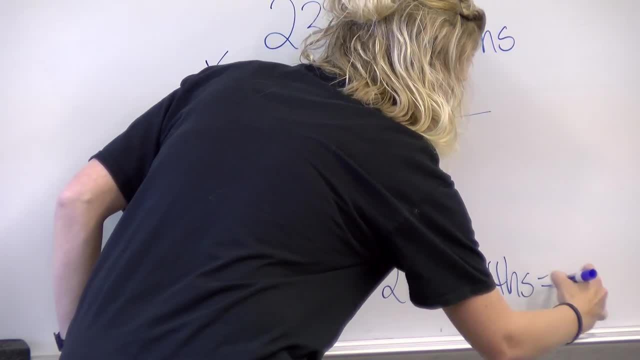 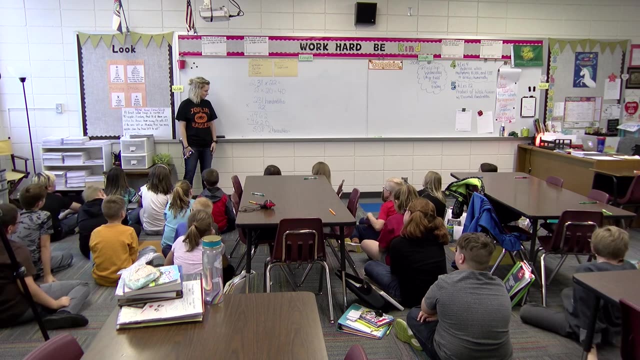 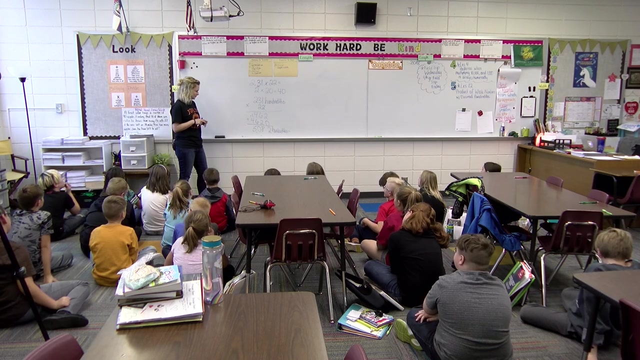 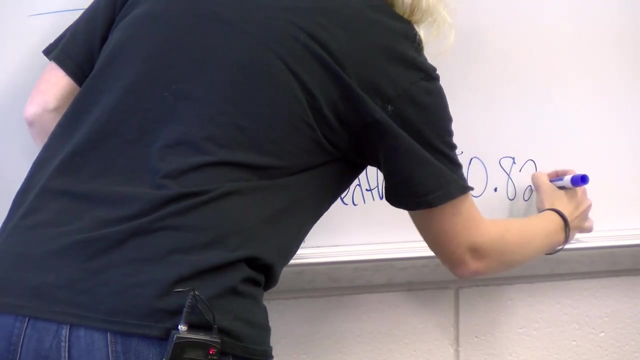 form. I need it expressed in standard form. Can someone tell me What does that mean? Oh, we put it back in. Okay, So where would the decimal go? Okay, I would agree. Raise your hand if you need me. 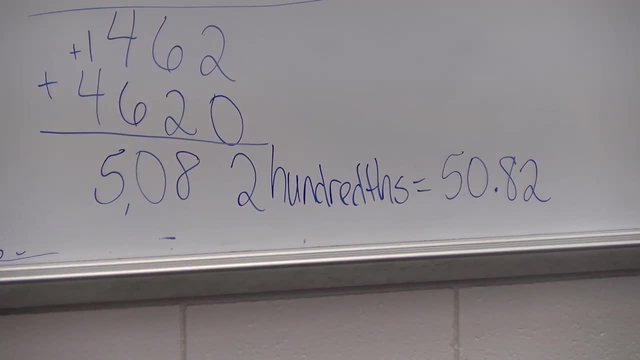 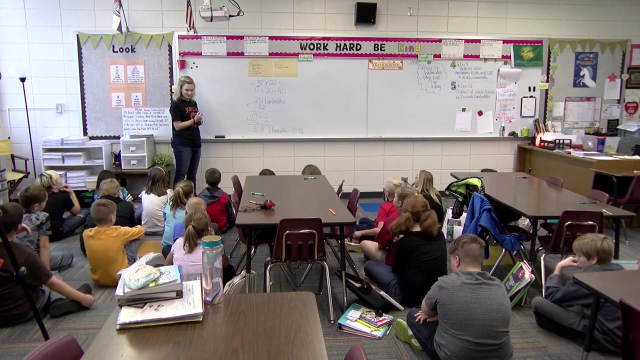 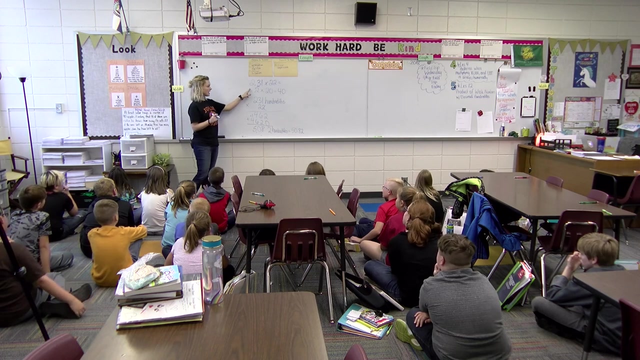 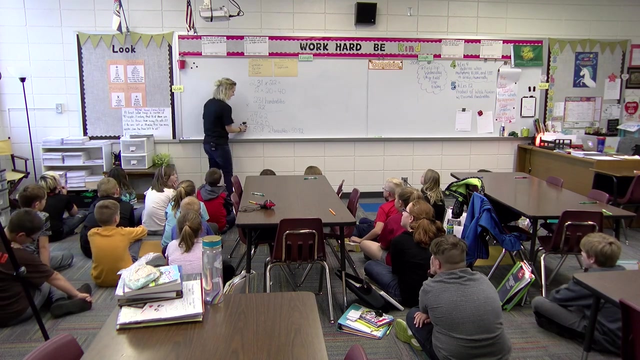 Yes, I like how that worked out for us. Questions you have right now on whether it's the estimating of the factors, renaming or the standard algorithm. Okay, Let's do another one. I like what I'm seeing with my participation. 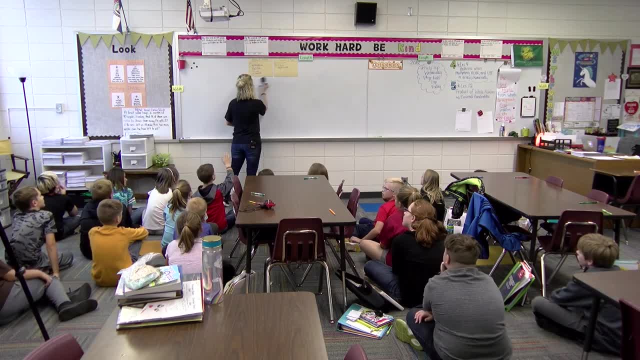 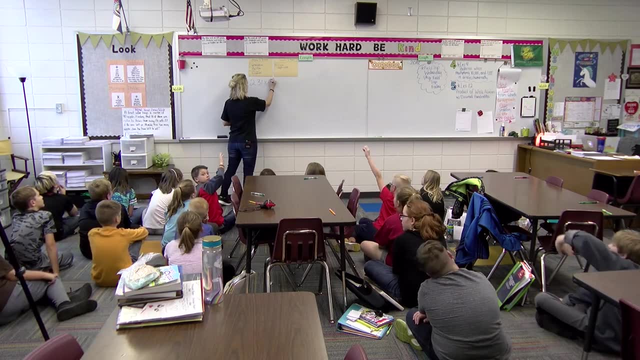 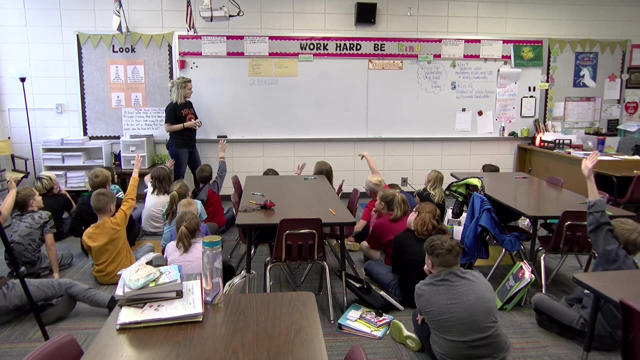 Keep it up, Okay. What do you guys notice about this problem compared to the last problem we just did? Mr Dunn, what do you think It's in the hundreds place? This one's in the hundreds place. What place was it in before? 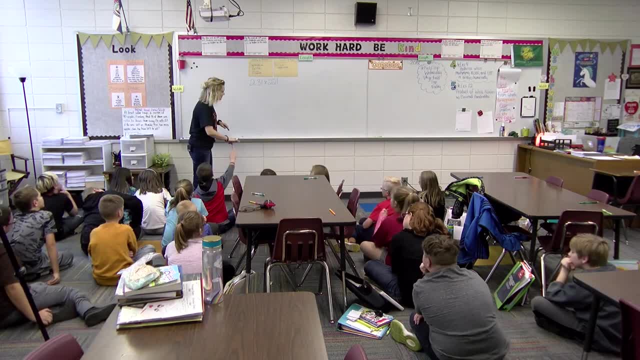 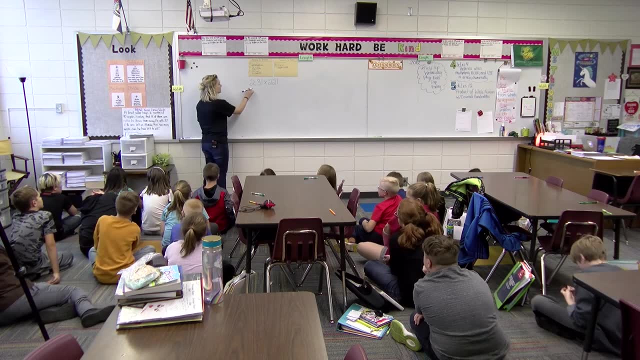 It was in the tenths place. High five it. Yes, Good job. Now I need someone to help me with my estimation of factors. Who would like to assist Cole? Okay, So two in thirty-one hundreds. What are we going to round that to? 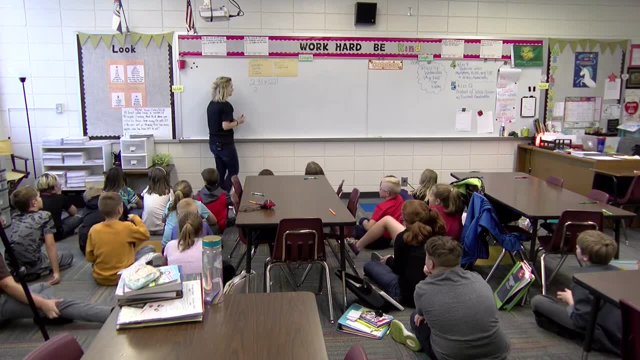 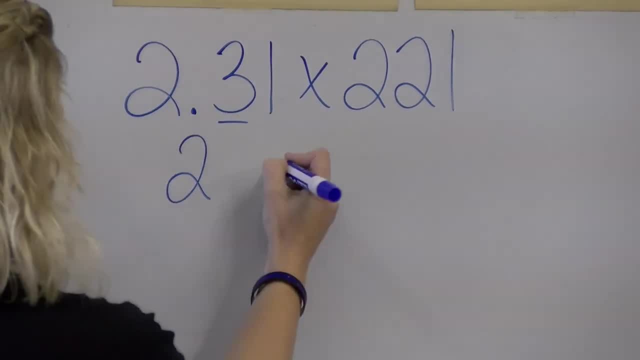 Two. How did you know we're rounding it just to two? Because when you go in the tenths place it is below five, so we round down. Okay, Keep going with it, Cole. Now you could go two different ways with this next factor, Cole. 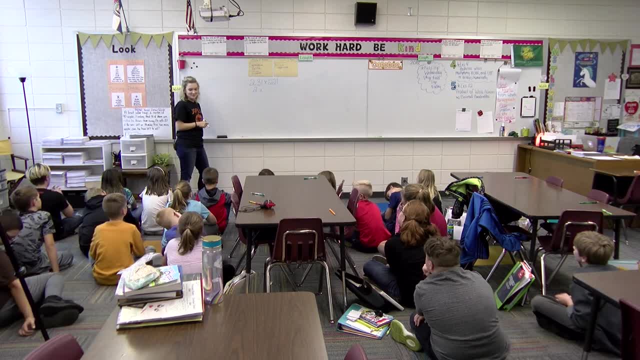 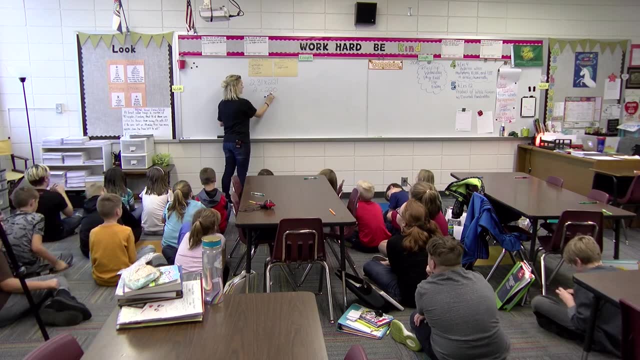 Can you express both ways? So you could do twenty, two hundred, twenty or just two hundred. So you rounded to: what place in this Round? What place value? Um, Wait, what do you mean by that? What place value did you just round to? 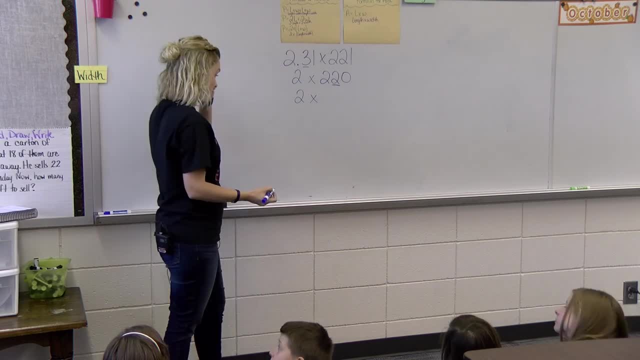 Oh, in the tenths, Okay. So if we express it in another way and you said two hundred, what place value did you round to in that expression? One hundred, Okay. Would I accept either, Yes, Yes, Unless it specifically tells you you could do either of these and they would be accepted. 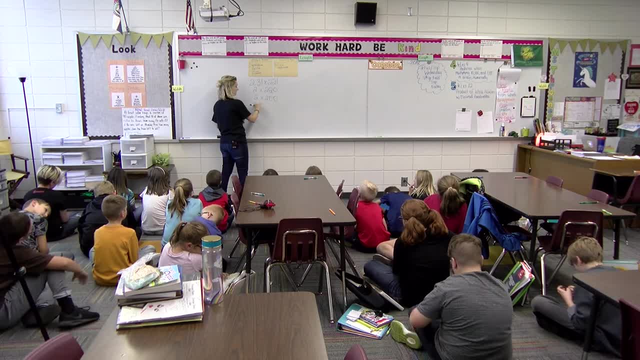 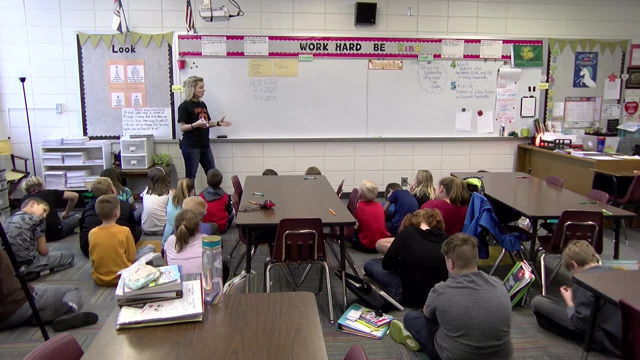 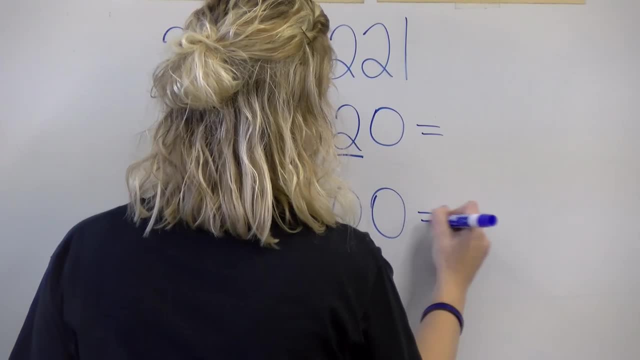 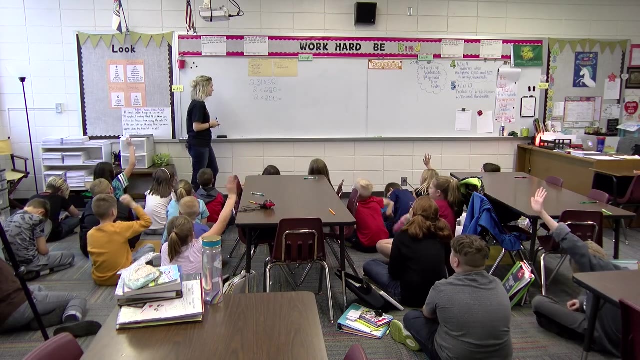 One hundred One hundred One hundred. Okay, Let's find the estimated product to both sets of estimated factors. Two times two hundred and twenty. What's the answer, Chloe? Four hundred and forty, Four hundred and forty Mm-hmm. 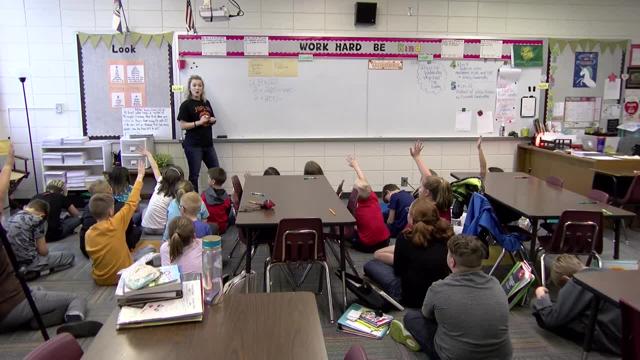 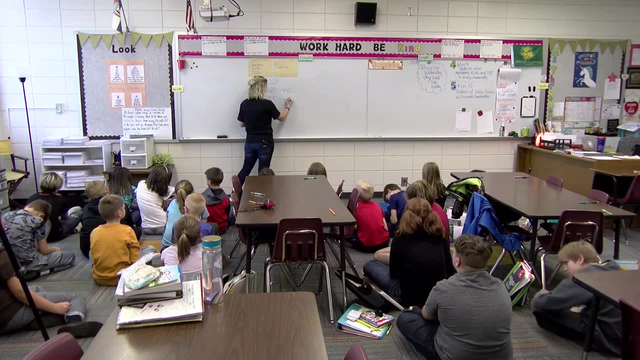 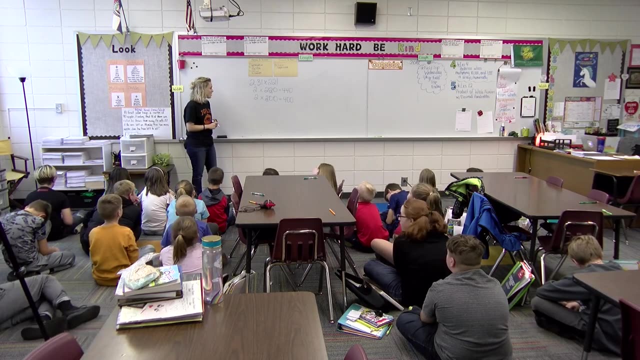 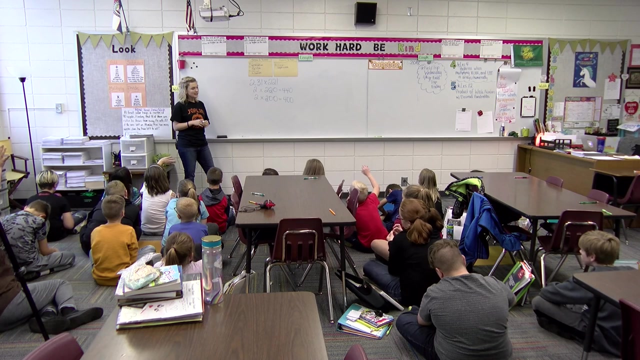 Two times two hundred, Alexis, Four hundred Four hundred Mm-hmm. Either of those would be accepted, because I could see your thinking either way. Okay, Now we now need to take and do a standard algorithm. What factors am I going to use for my standard algorithm? 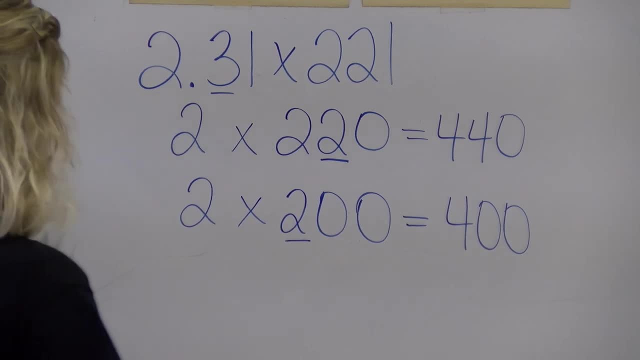 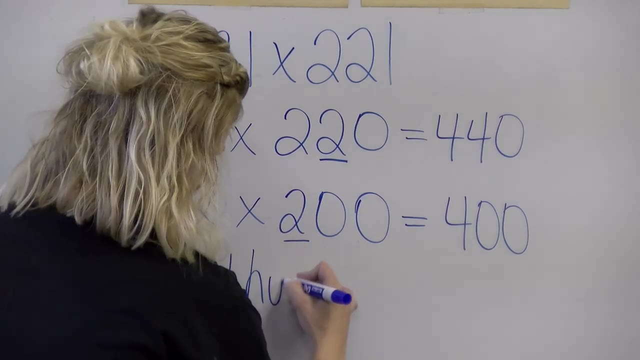 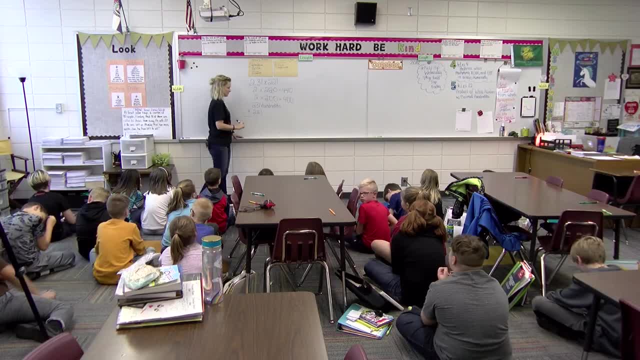 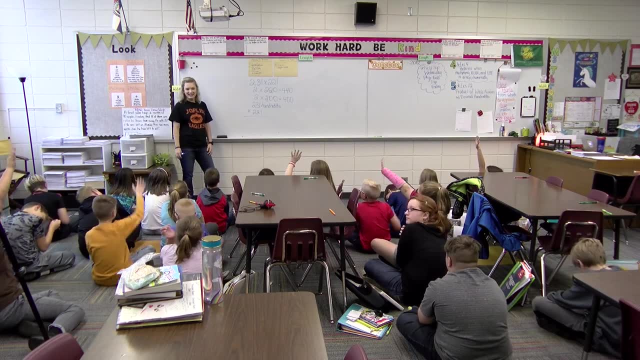 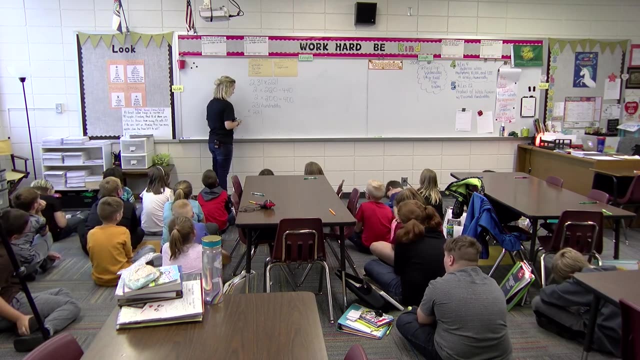 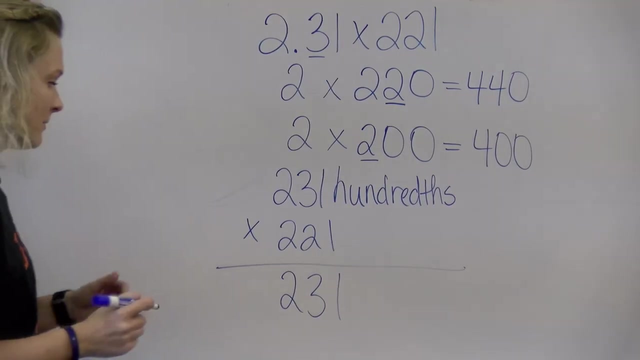 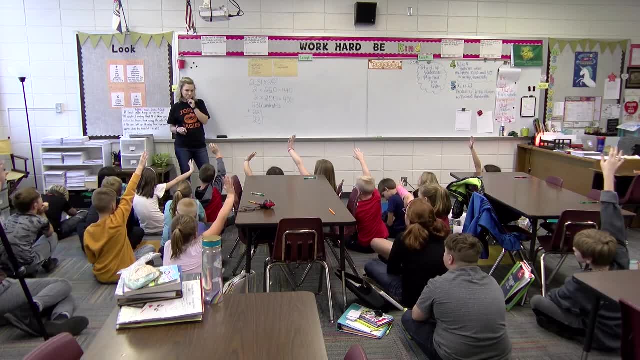 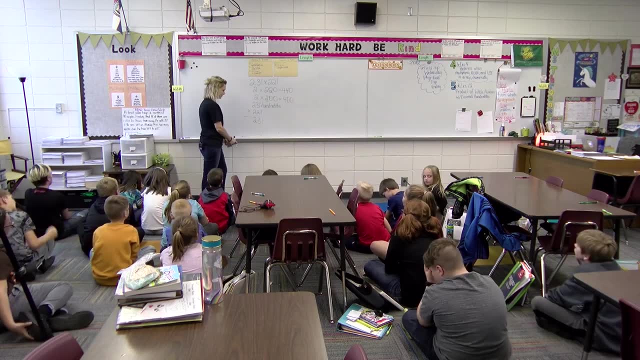 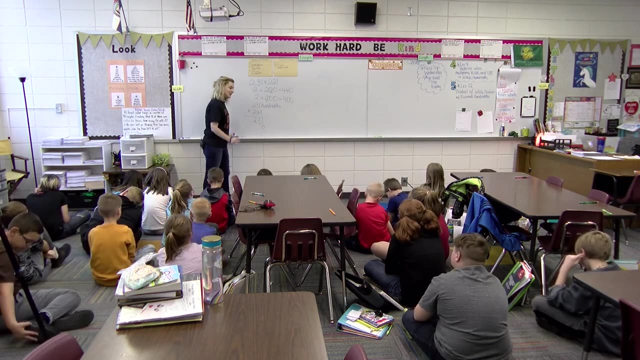 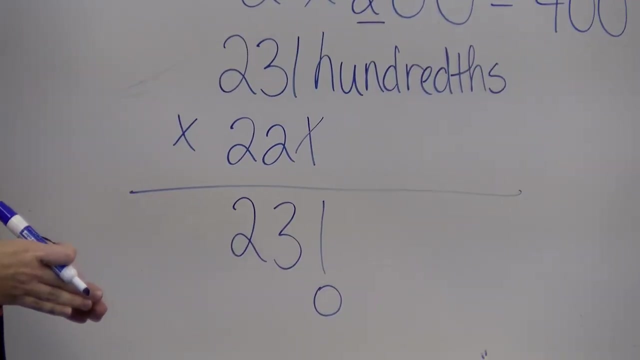 got to do something pretty important over here. hmm, Kaylee, when are you thinking put a zero where under the one? because that is, in what place value the ones? and we're done with the ones, right? so what place value are we going to go work with, Kaylee, the tens? thank you. so two times one, Jade, you're gonna help me. 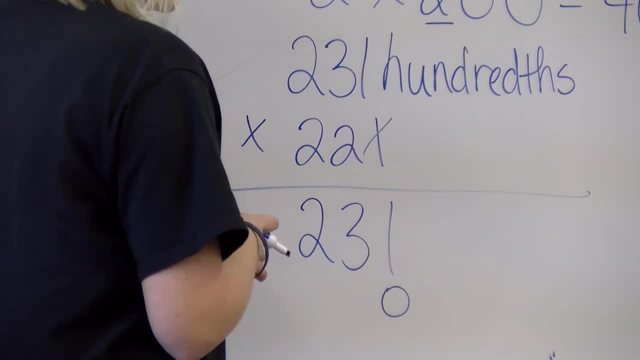 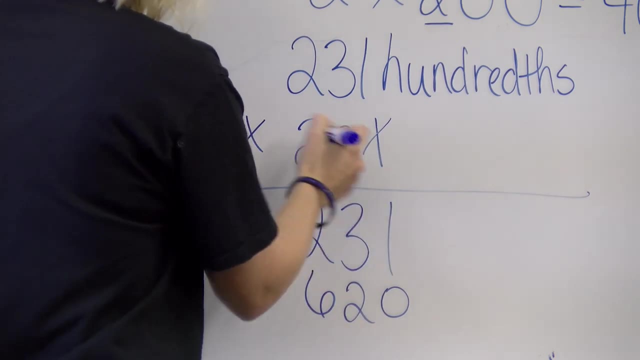 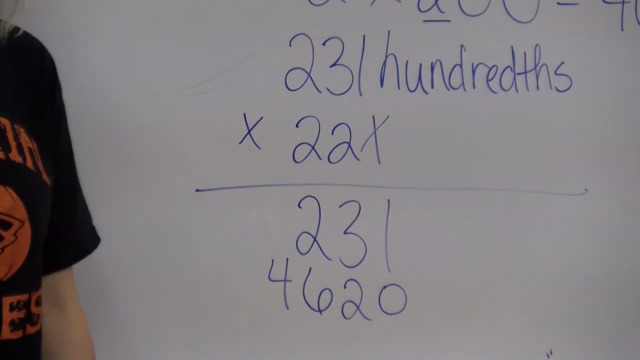 what's two times one? three, four, five, six, six, five, seven, seven, eight, nine, ten times 1, sweetheart 2. 2. 2 times 3, Jade 6. 2 times 2? 4.. Thank you, Now this one. 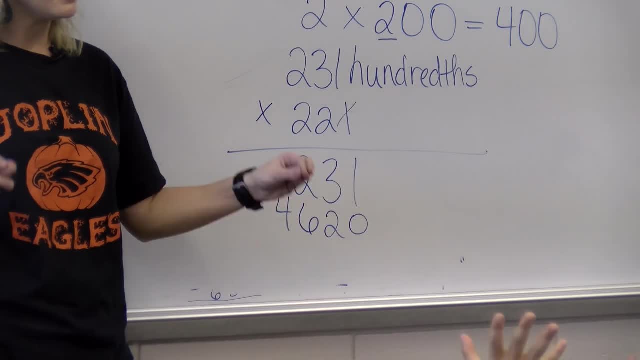 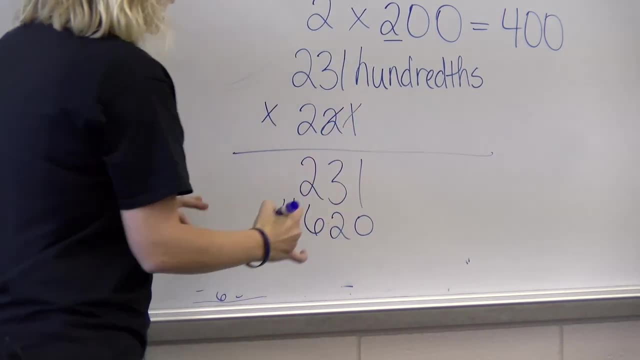 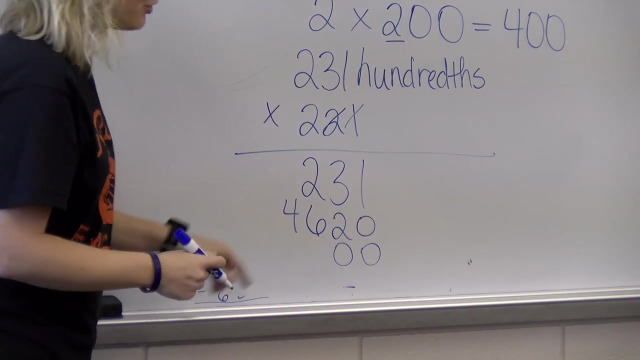 could get a little dicey. What do we still have to do? There's something really important we need to do here. Megan, I now have to put two zeros there. Okay, Megan, you have to explain. Why am I putting two zeros on that third row of multiplication? Remember those. 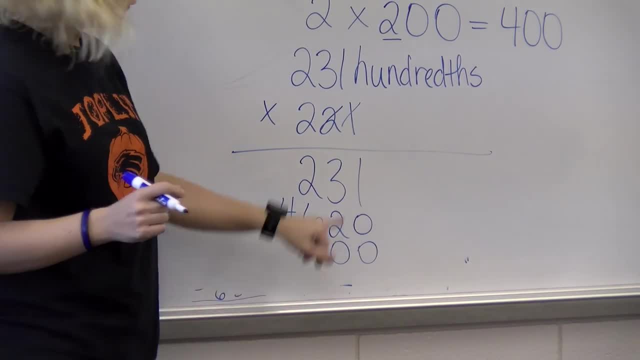 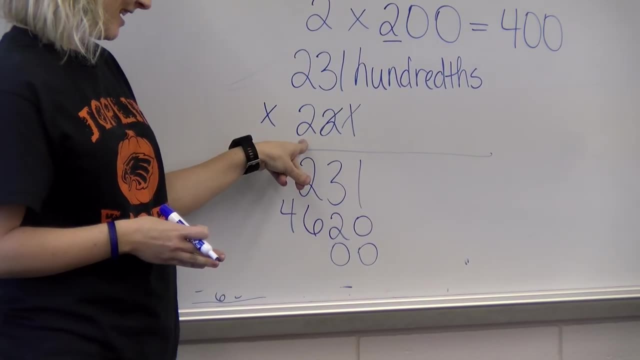 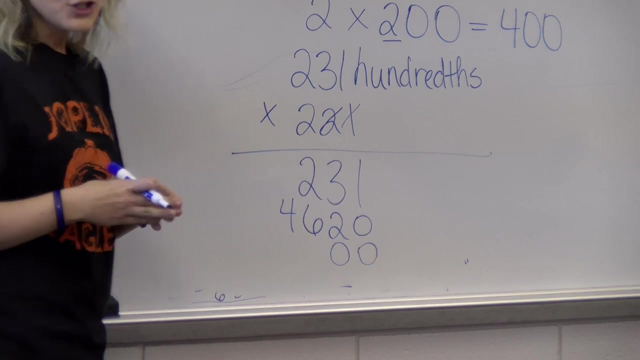 zeros. tell your brain what you've already done. multiplication-wise, You've dealt with the ones place, the tens place. now, what place are we going to work in? Hundreds, Hundreds. You're good. thank you, Alright. who would like to help me finish? 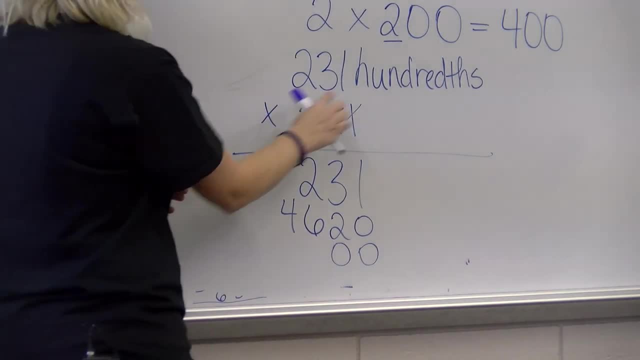 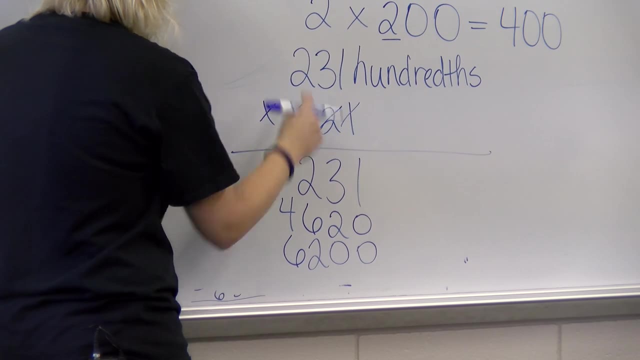 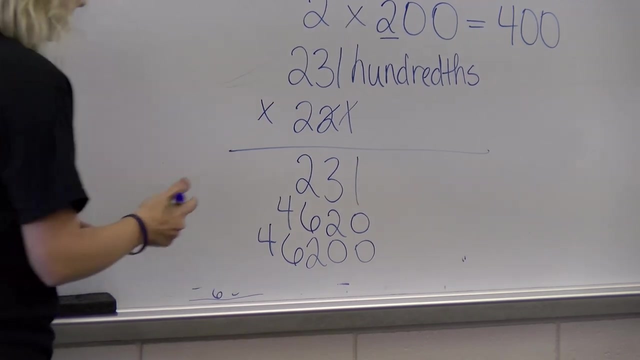 it out here: Elena: 2 times 1? 2.. 2 times 3? 6. 2 times 2? 4. Elena, now that we're done with our multiplication, what can we do? Add, Add. We're going to add up these partial products.